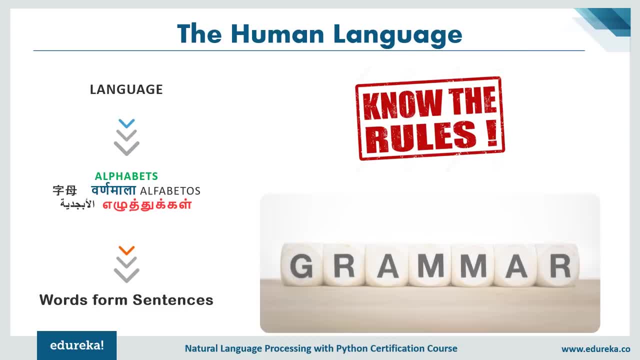 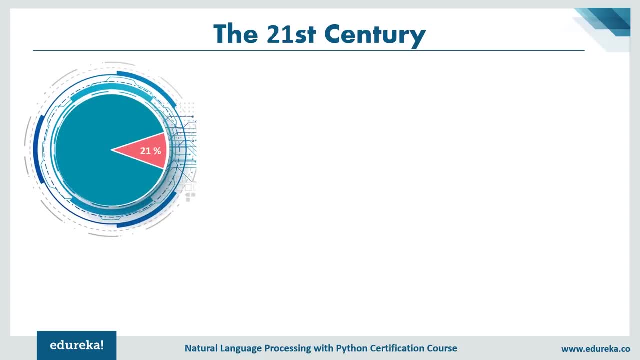 while developing these sentences and these set of rules are also known as grammar. Now, coming to today's world, that is, the 21st century, according to the industry estimates, only 21% of the available data is present in the structured format. Data is being generated as we speak, as we tweet, as we send. 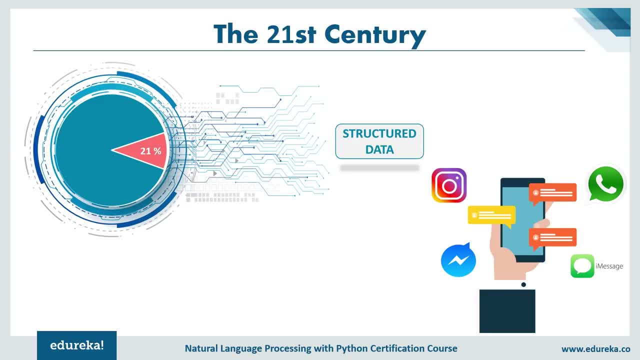 messages on whatsapp, facebook, instagram or through text messages, and the majority of this data exists in the textual form, which is highly unstructured in nature. Now, in order to produce significant and actionable insights from the text data, it is important to get acquainted with the techniques of text and language processing Now in order to produce significant and actionable insights from. 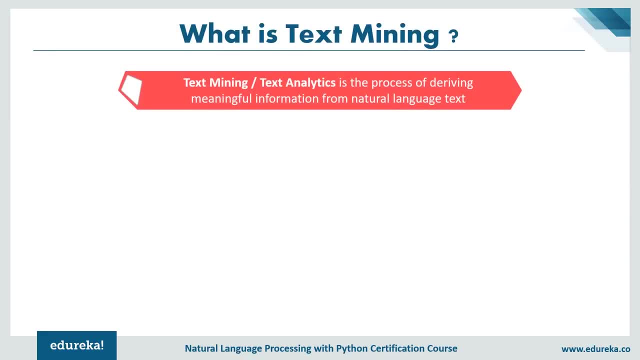 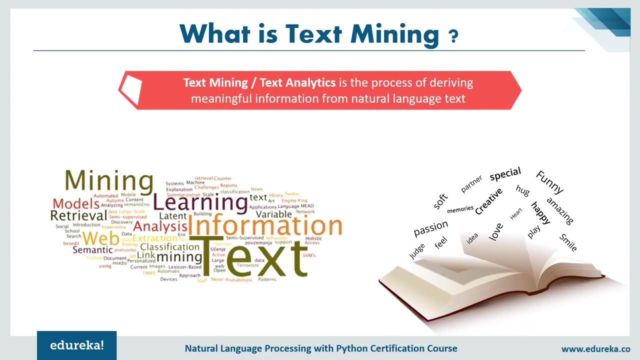 text analysis. So let's understand what is text analysis or text mining Now. it is the process of deriving meaningful information from natural language text, and text mining usually involves the process of structuring the input text, deriving patterns within the structured data and finally evaluating the interpreted output Compared with the kind of data stored in database. text is 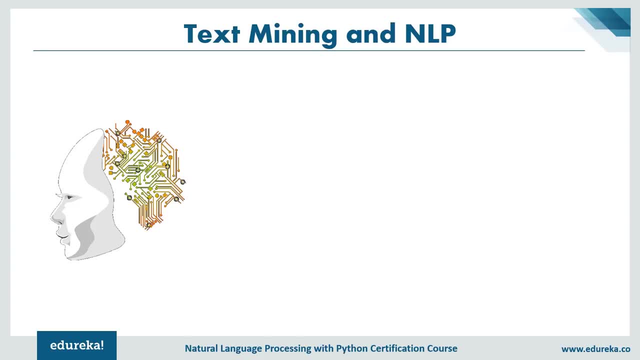 unstructured, amorphous and difficult to deal with algorithmically. Nevertheless, in the modern culture, text is the most common source of information, and it is the most common source of information Now, as text mining refers to the process of deriving high quality information from text, the overall goal, 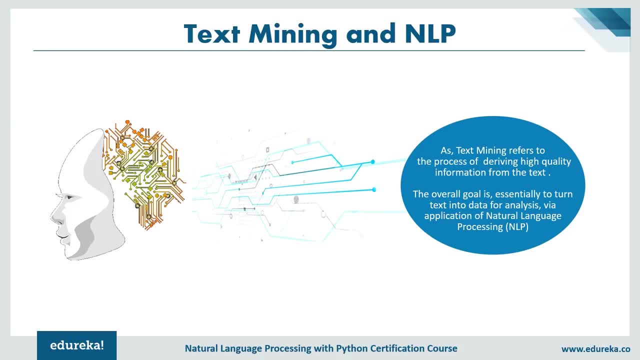 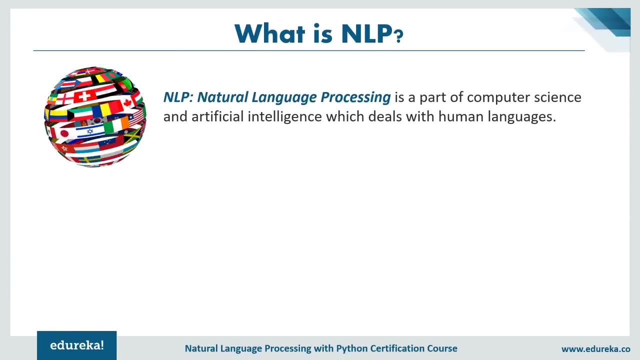 here is to turn the text into data for analysis, and this is done by the application of NLP or natural language processing. So let's understand what is natural language processing. So NLP refers to the artificial intelligence method of communicating with an intelligent system using natural language. 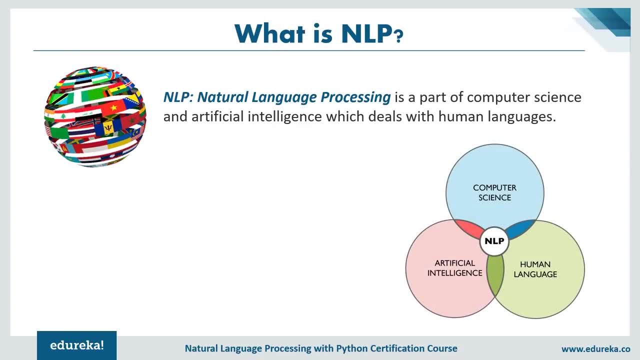 by utilizing NLP. So NLP refers to the artificial intelligence method of communicating with an intelligence system using natural language by utilizing NLP. So NLP refers to the artificial intelligence method of communicating with an intelligent system using natural language by utilizing NLP and its components. 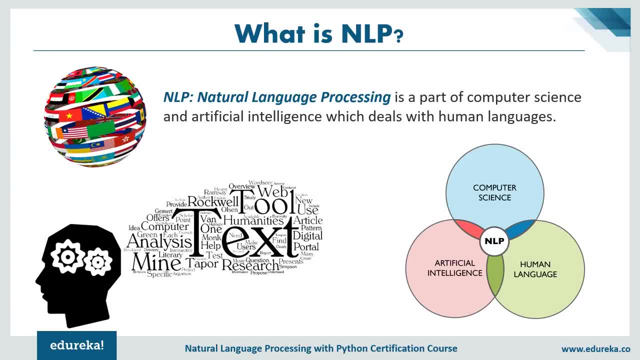 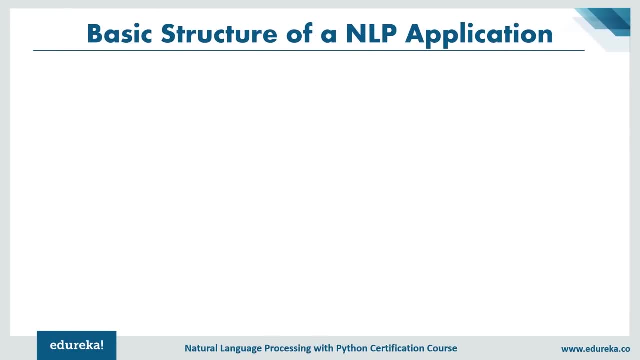 One can organize the massive chunks of textual data, perform numerous or automated task and solve a wide range of problems such as automatic summarization, machine translation, name entity recognition, speech recognition and topic segmentation. So let's understand the basic structure of an NLP application. considering the chat bot here as an example, we can see: 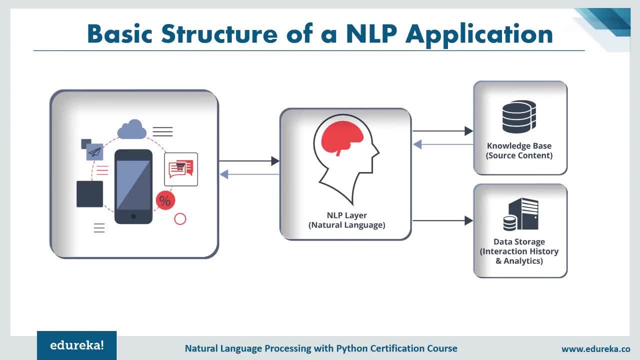 First we have the NLP layer, which is connected with the knowledge base and the data storage. Now the knowledge base is where we have the source content, that is, we have all the chat logs, which contain a large history of all the chats which are used to train the particular algorithm, and again we have the data. 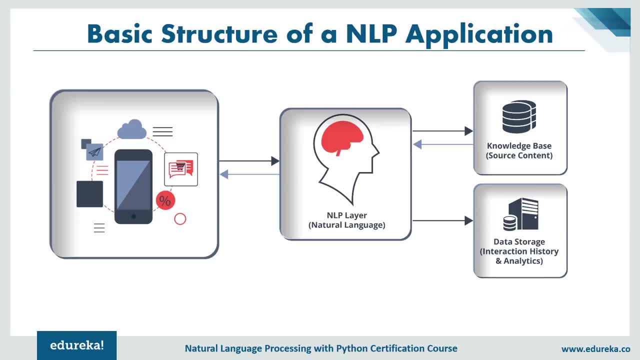 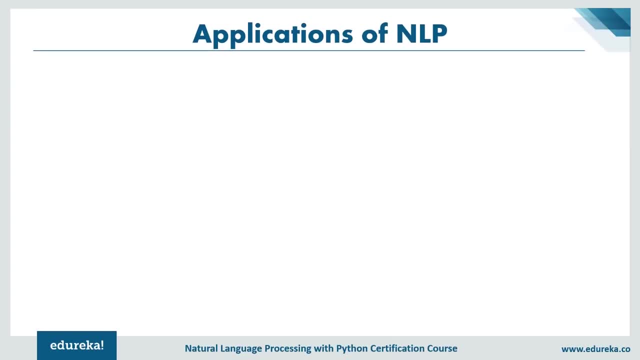 storage, where we have the interaction history and the analytics of that interaction, which in turn helps the NLP layer to generate the meaningful output. So now, if we have a look at the various applications of NLP, first of all we have sentimental analysis. now this is a field where NLP is used. 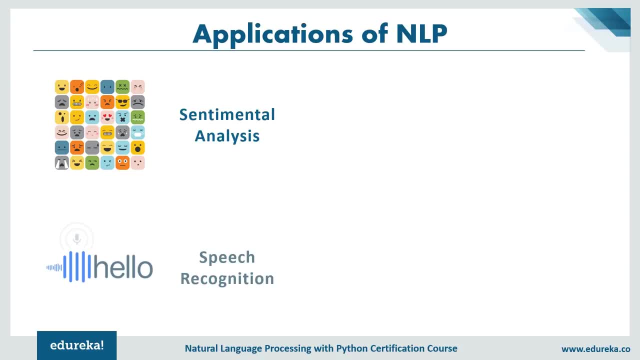 heavily. we have speech recognition now. here we are also talking about the voice assistants, like Google Assistant, Cortana and the Siri. Now. next, we have the implementation of chatbot, as I discussed earlier, just now. Now you might have used the customer care chat services of any app. it also 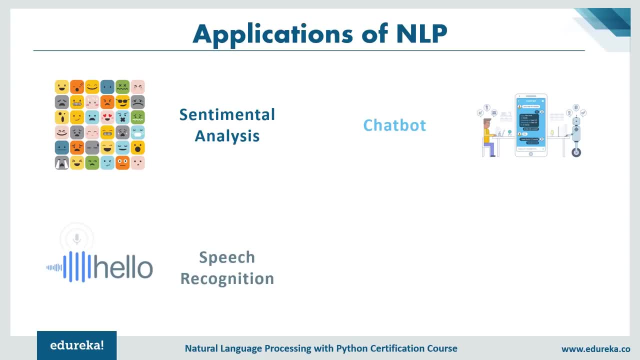 uses NLP to process the data entered and provide the response based on the input. Now, machine translation is also another use case of natural language processing. Now, considering the most common example here would be the Google Translate. It uses NLP and translates the data from one language to another, and that, too, in real time. 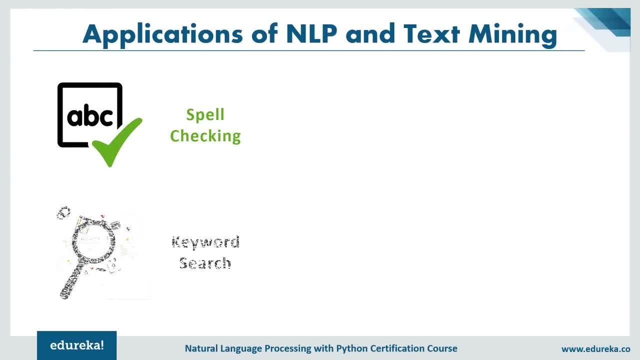 Now, other applications of NLP includes spell checking. then we have the keyword search, which is also a big field where NLP is used. extracting information from any particular website or any particular document is also a use case of NLP, and one of the coolest application of NLP is advertisement. 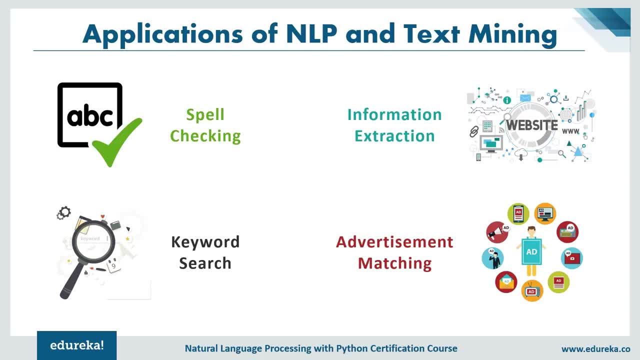 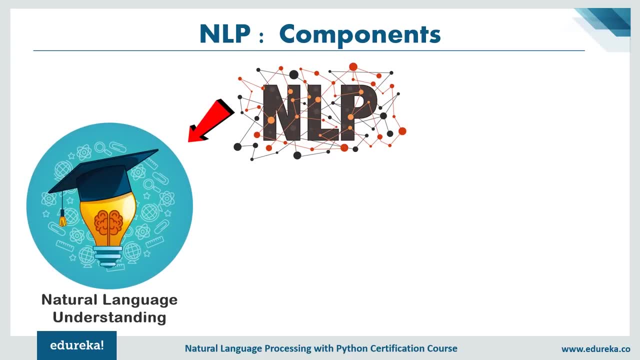 matching. Now, here, what we mean is basically recommendation of the ads based on your history. Now NLP is divided into two major components. that is, the natural language understanding, which is also known as NLU, and we have the natural language generation, which is also known as NLG. 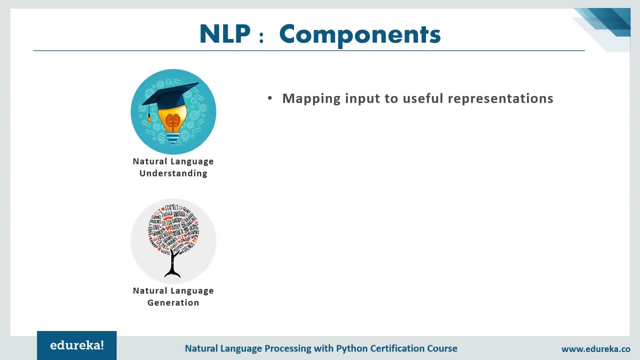 The understanding involves tasks like mapping the given input into natural language into useful representations, analyzing different aspects of the language. whereas natural language generation, it is the process of producing the meaningful phrases and sentence in the form of natural language, It involves text planning, sentence planning and text realization. now NLU is usually considered harder than NLG. now, 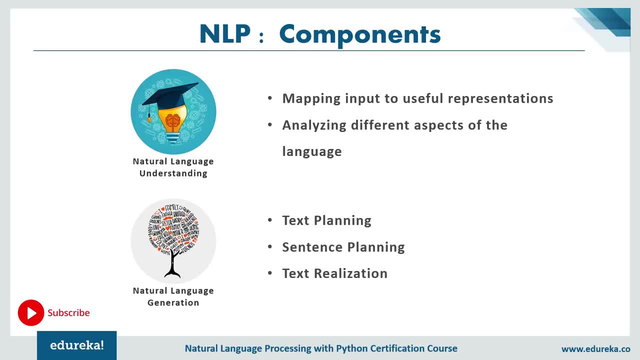 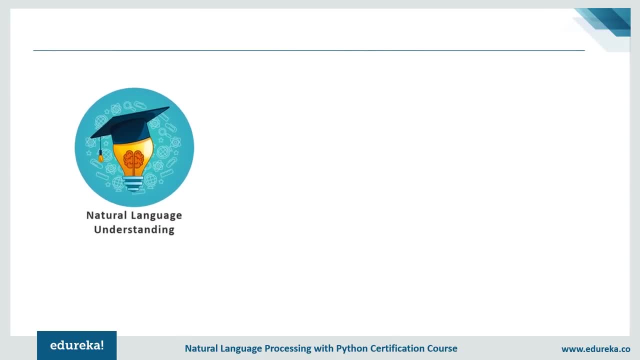 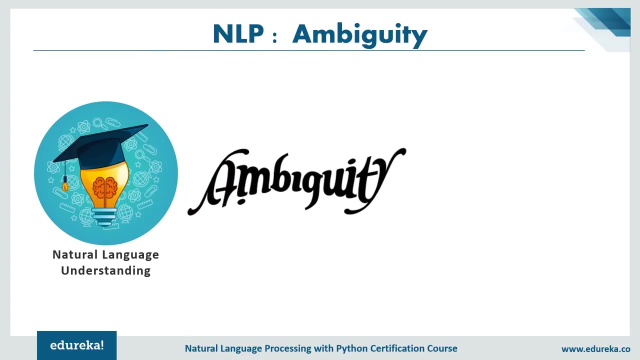 you might be thinking that even a small child can understand a language, So let's see What are the difficulties a machine faces while understanding any particular languages. now, understanding a new language is very hard. taking our English into consideration, There are a lot of ambiguity, and that, too, in different levels. 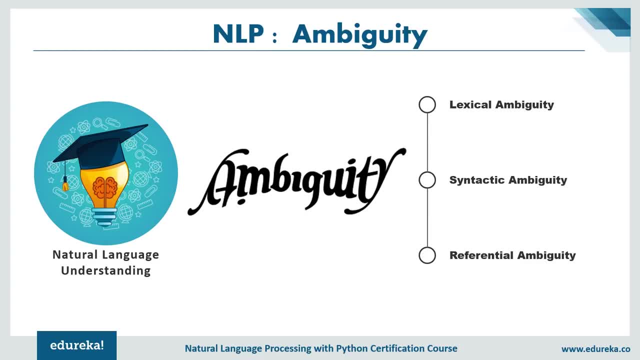 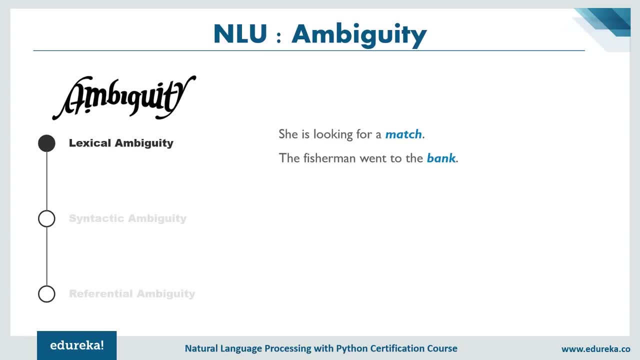 We have lexical ambiguity, syntactical ambiguity and referential ambiguity. So lexical, Ambitious. Ambitious: the presence of two or more possible meanings within a single word. It is also sometimes referred to as semantic ambiguity, For example. let's consider these sentences and let's focus. 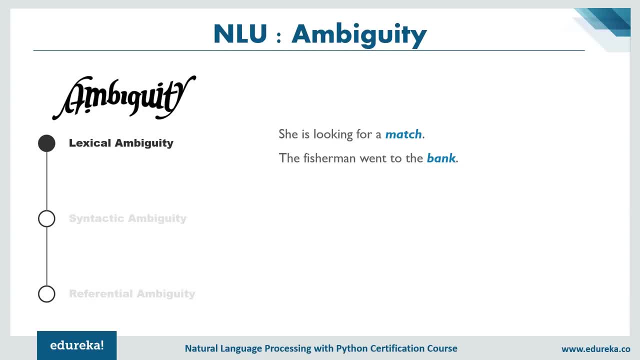 on the italicized words: She is looking for a match. So what do you infer by the word match? Is it that she's looking for a partner, or is it that she's looking for a match, be it a cricket match or a rugby match? Now the second sentence here we have: the fisherman went to the bank. 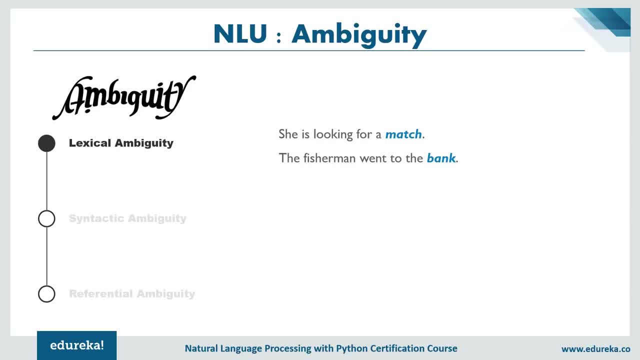 Is it the bank where we go to collect our checks and money, or is it the river bank we are talking about here? Sometimes it is obvious that we are talking about the river bank, but it might be true that he's actually going to a bank to withdraw some money, You never know. Now, coming to the 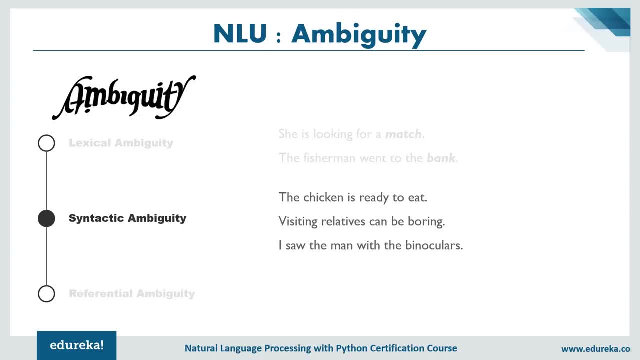 second type of ambiguity, which is the syntactical ambiguity. In English grammar, this syntactical ambiguity is the presence of two or more possible meanings within a single sentence or a sequence of words. It is also called a structural ambiguity or grammatical ambiguity. Taking these sentences into consideration, we can clearly see what are the ambiguities faced. 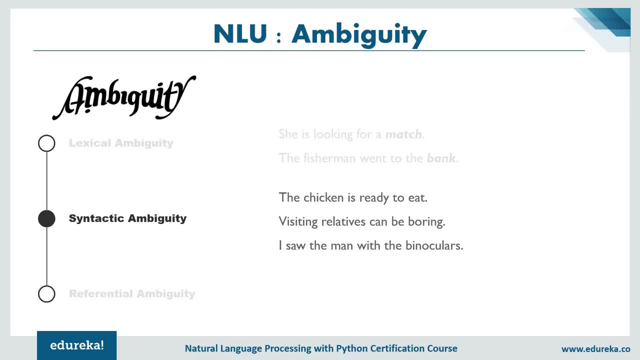 The chicken is ready to eat. So here, what do you infer? Is the chicken ready to eat his food, or is the chicken ready for us to eat? Similarly, we have the sentence: like visiting relatives can be boring, Are the relatives boring? or when we are visiting the relative, it is very boring, You never. 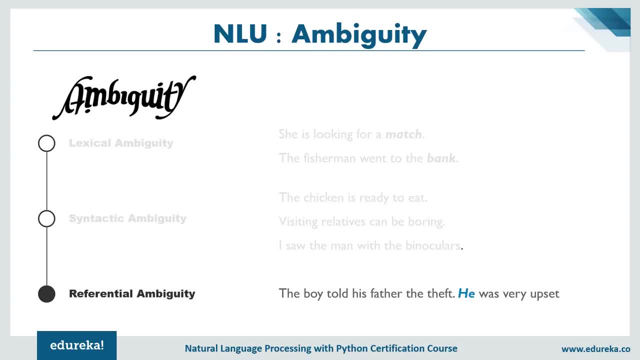 know Coming to the final ambiguity, which is the referential ambiguity. Now this ambiguity arises when we are referring to something using pronouns. The boy told his father the theft. He was very upset. Now I'm leaving this up to you. You tell me. 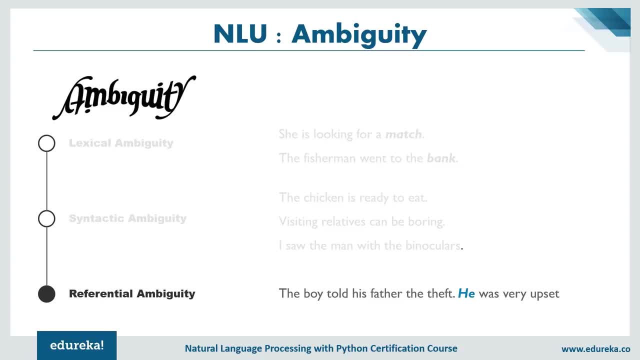 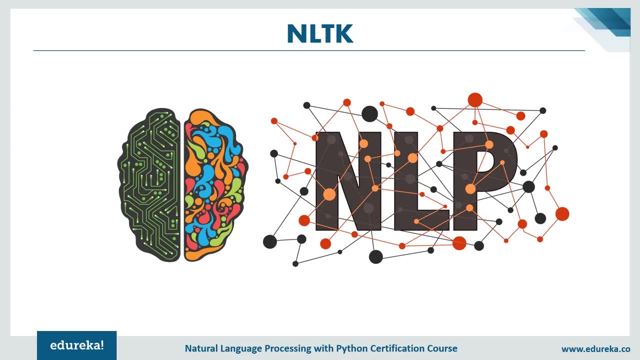 what does he stand for here? Who is he? Is it the boy, Is it the father or is it the thief? So, coming back to NLP, firstly we need to install the NLTK library, that is, the natural language toolkit. It is the leading platform for building Python programs to work with human. 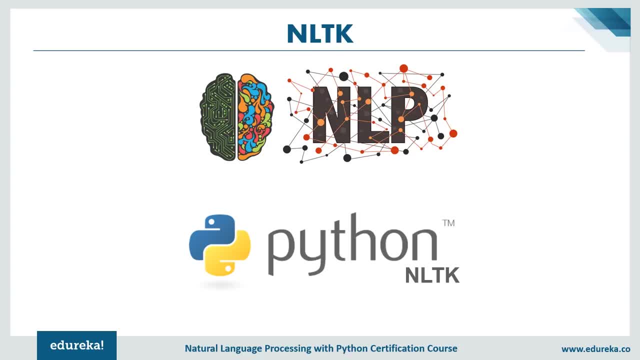 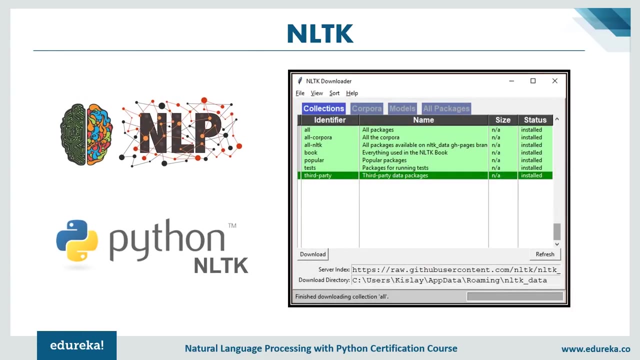 language data, and it also provides easy to use interfaces to over 15 corpora and lexical sources. We can use it to perform functions like classification, tokenization, stemming, tagging and much more. Now, once you install the NLTK library, you will see an NLTK downloader. It is a pop-up. 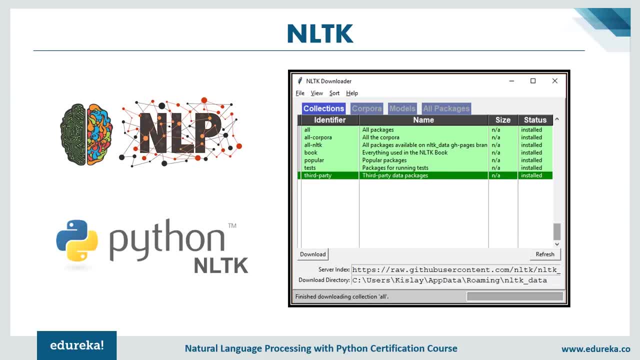 window It will come up and in that you have to select the all option and press the download button. It will download all the required files: the corpora, the models and all the different packages which are available in the NLTK. Now, when we process text, there are a few terminologies. 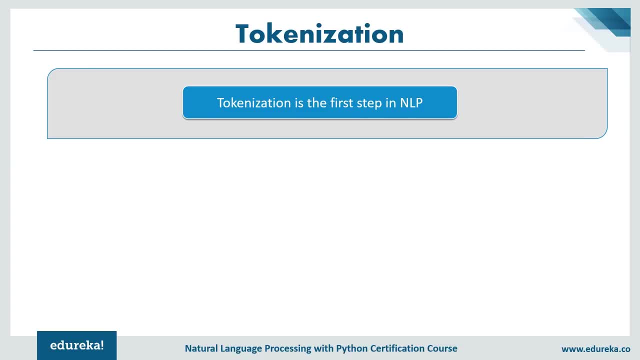 that we need to understand Now. the first one is tokenization. So tokenization is a process of breaking strings into tokens, which in turn, are small structures or units that can be used for tokenization. Now tokenization involves three steps, which is breaking a complex sentence into. 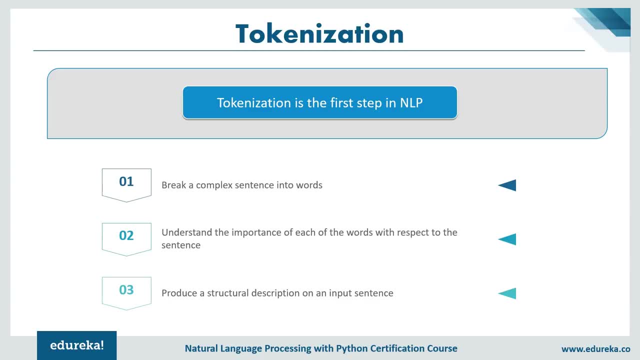 words, understanding the importance of each words with respect to the sentence and finally produce a structural description on an input sentence. So if we have a look at the example here, considering this sentence, tokenization is the first step in NLP. Now, when we divide it into tokens, as you can see, here we have 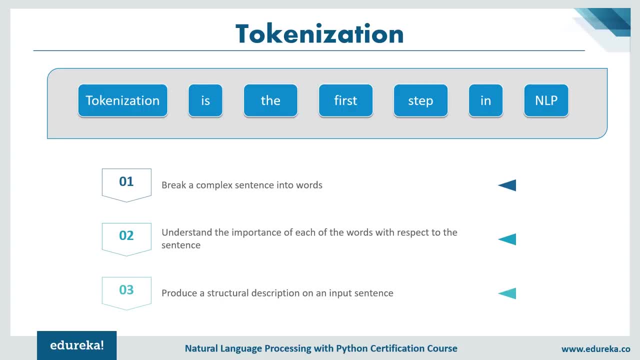 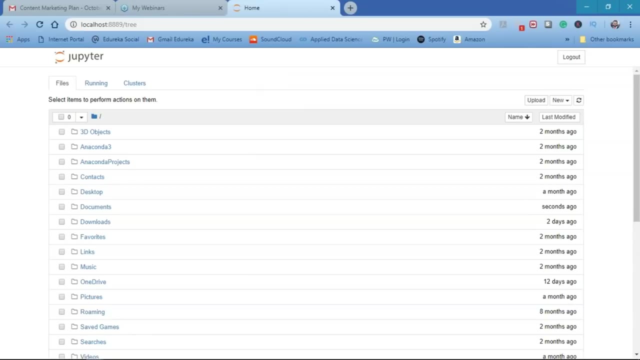 one, two, three, four, five, six and seven tokens here. Now NLTK also allows you to tokenize phrases containing more than one word, So let's go ahead and see how we can implement tokenization using NLTK. So here I'm, using Jupyter notebook to execute all my practicals and demo. Now you are free to. 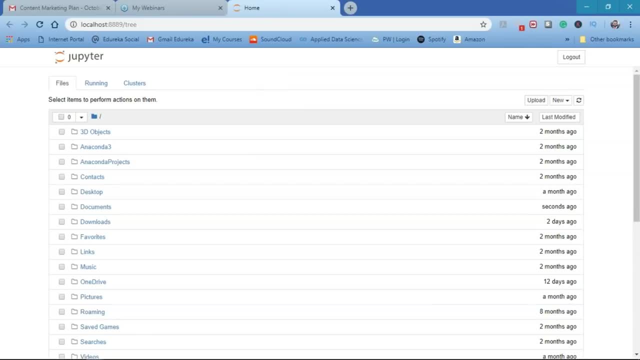 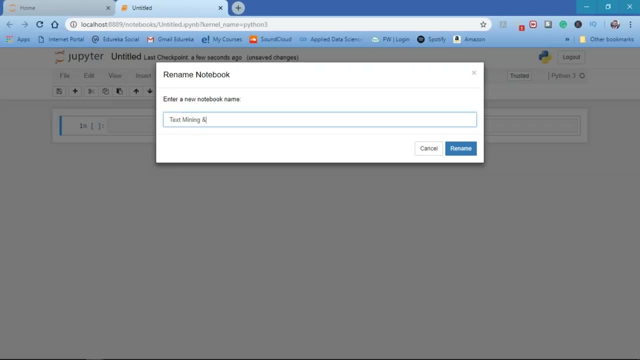 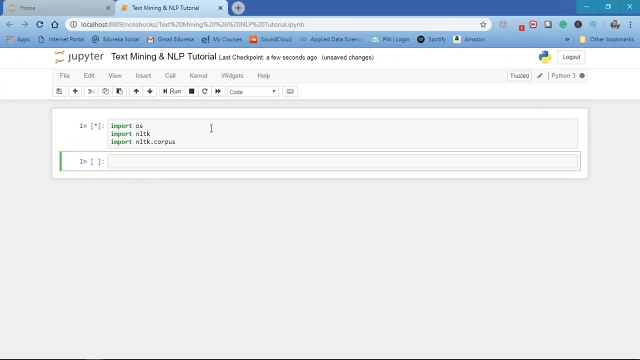 use any sort of IDE which is supported by Python. It's your choice. So let me create a new notebook that we rename as Text Mining and NLP. So first of all, let us import all the necessary libraries. here We are importing the OS, NLTK and 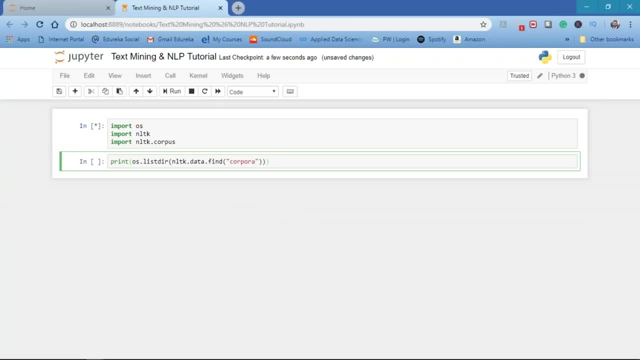 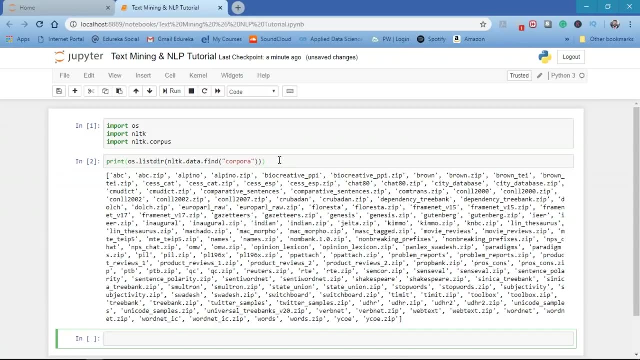 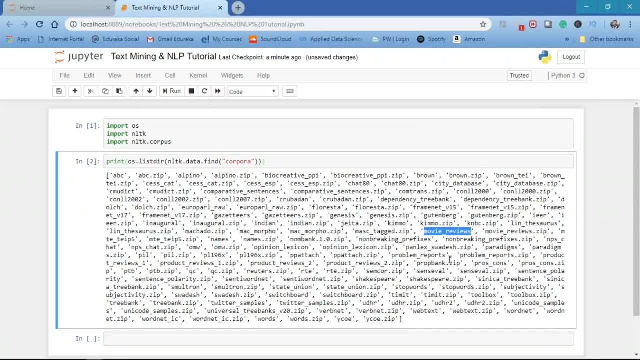 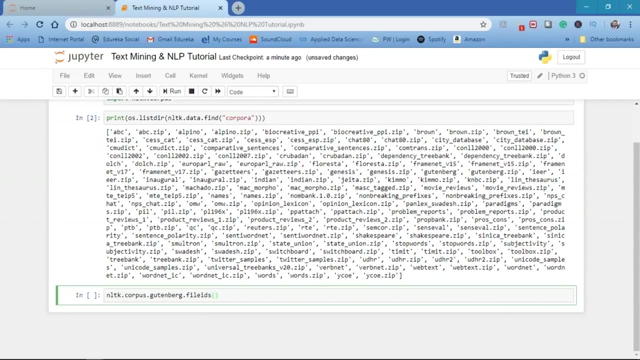 reviews, We have movie reviews, We have non-breaking prefixes and many more files here. Now let's have a look at the Gutenberg file here and see what are all the fields which are present in the Gutenberg file. So, as you can see, here inside this we have all the different types of 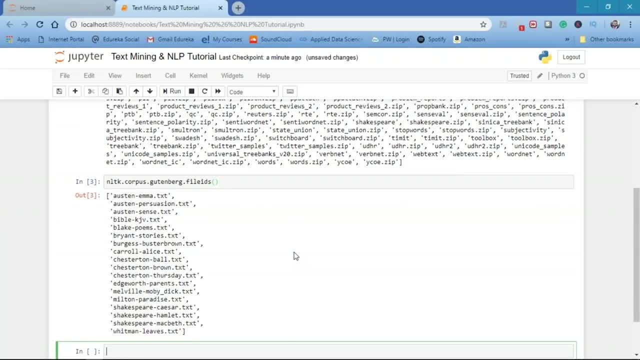 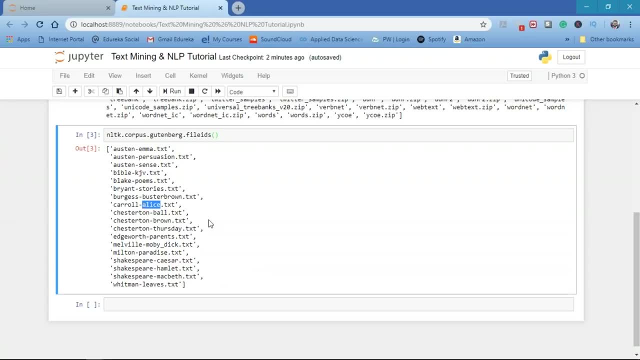 text files. We have Austin Emma, We have the Shakespeare, We have the Hamlet, We have Moby Dick's, We have the Carol, Alice and many more. Now this is just one file we are talking about, and NLTK provides a lot of files, So let's consider a. 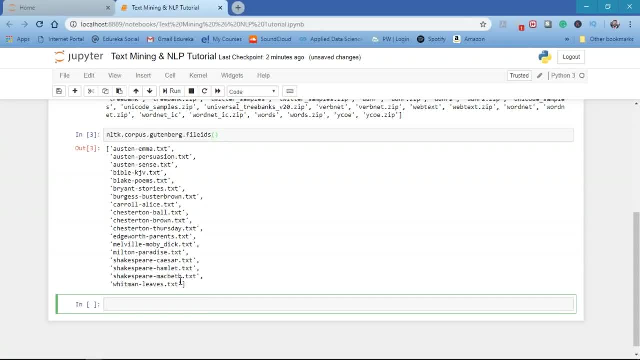 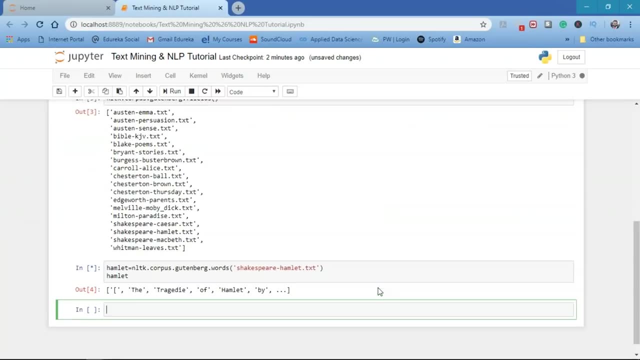 document of type string and understand the significance of its tokens. So if we have a look at the elements of the Hamlet, you can see it starts from the tragedy of Hamlet by William Shakespeare. So if you have a look at the first 500 elements of this particular text file, so, as I 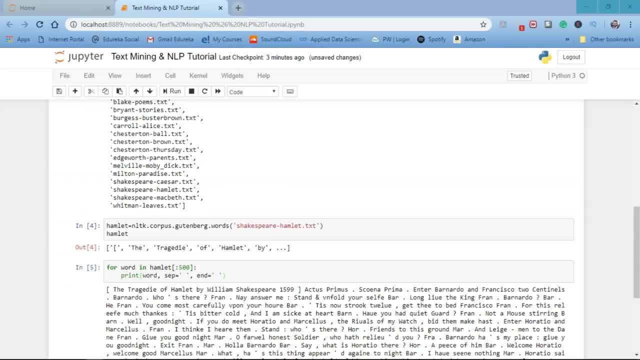 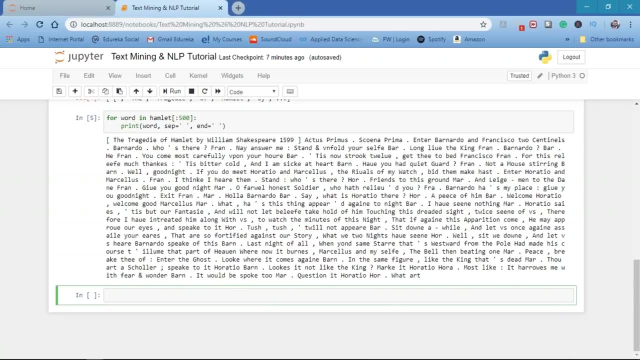 was saying the tragedy Hamlet by William Shakespeare 1597.. Actus Primus: We can use a lot of these files for analysis and text for understanding and analysis purposes, and this is where NLTK comes into picture and it helps a lot of programmers to learn about the different. 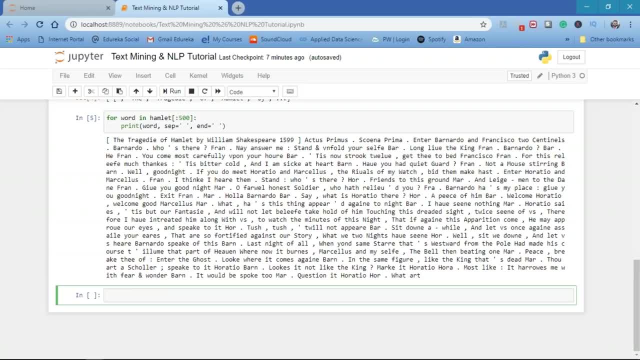 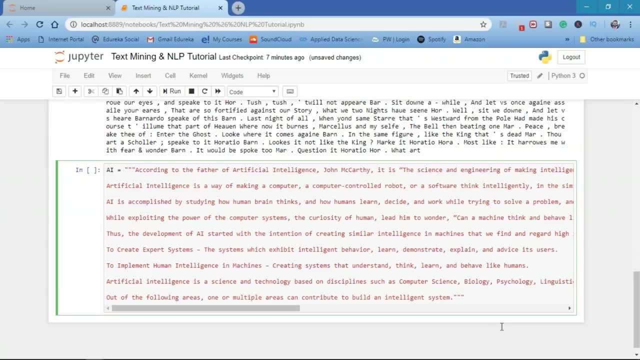 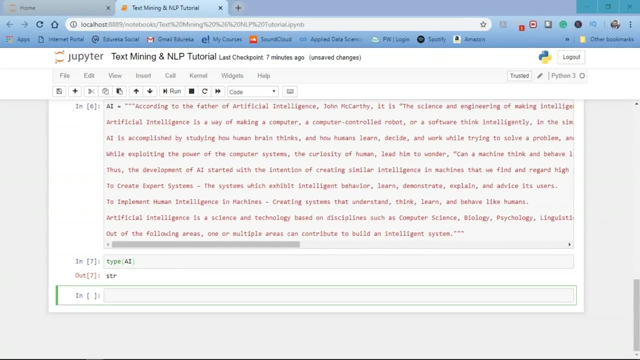 features and a different application of language processing. So here I have created a paragraph on artificial intelligence, so let me just execute it Now. this AI is of the string type, so it will be easier for us to tokenize it. Nonetheless, any of the files can be used to tokenize For simplicity. here I am. 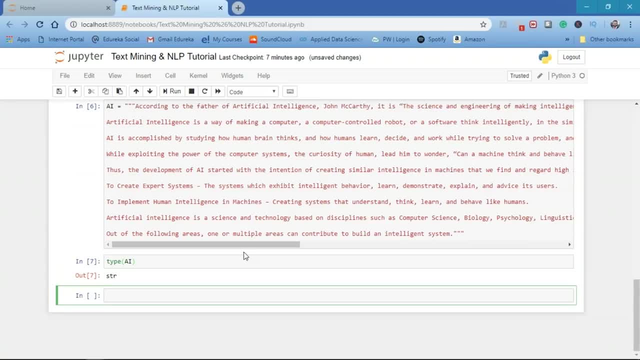 taking a string file. Next, what we are going to do is import the word underscore tokenize under the NLTK tokenize library. Now, this will help us to tokenize all the words. Now we will run the word underscore tokenize function over the paragraph and assign it a name. So here I am considering AI. 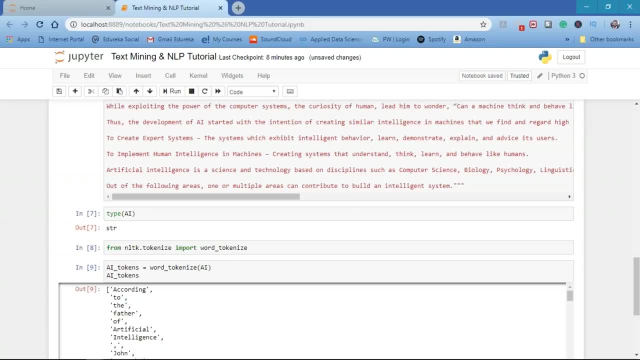 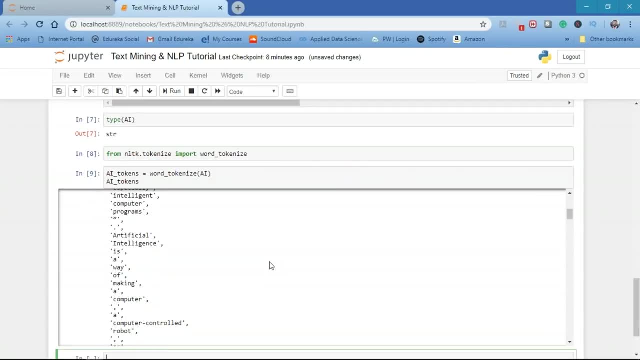 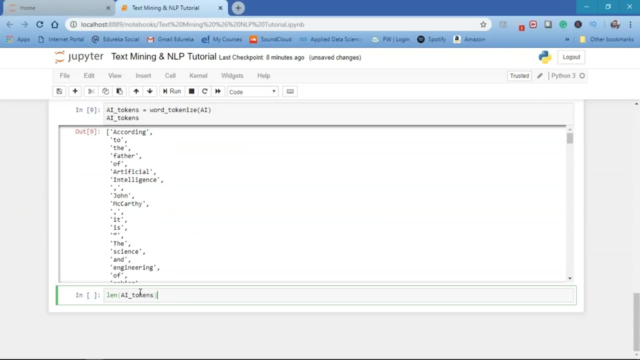 underscore tokenize. I'm using the word underscore tokenize function on it. Let's see what's the output of this AI: underscore tokens. So, as you can see here, it has divided all the input which was provided here into the tokens. Now let's have a look at the number of tokens here we have here. So in total we 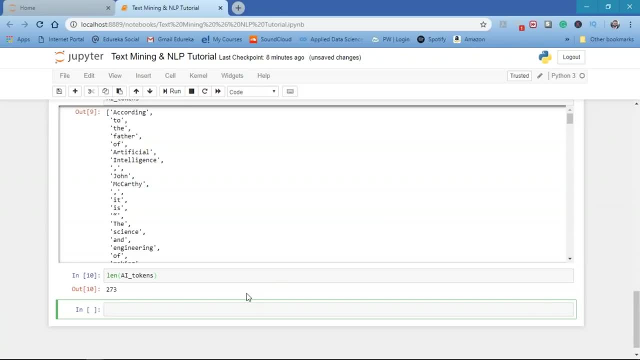 have 273 tokens Now. these tokens are a list of words and the special characters, which are separated items of the list. Now, in order to find the frequency of the distinct elements here in the given AI paragraph, we are going to import the frequency distinct function which falls under NLTK dot. 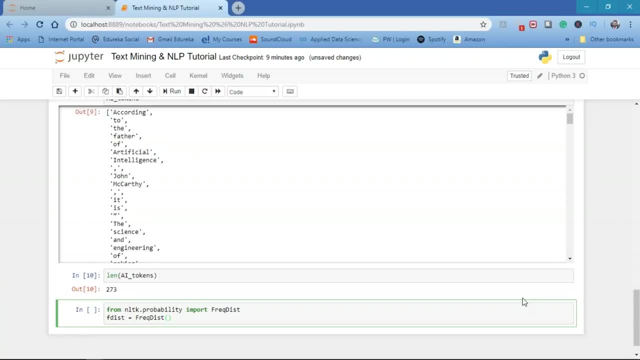 probability. So let's create a fdist in which we have the function here frequentist, and basically what we are doing here is finding the word count of all the words in the paragraph. So, as you can see, here we have comma 30 times. we. 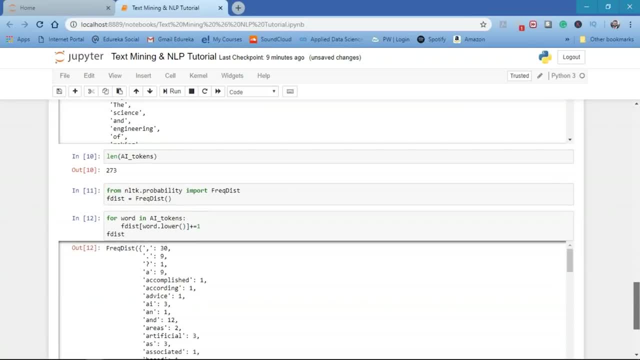 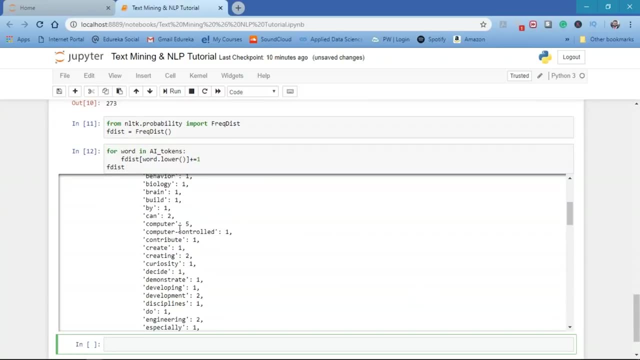 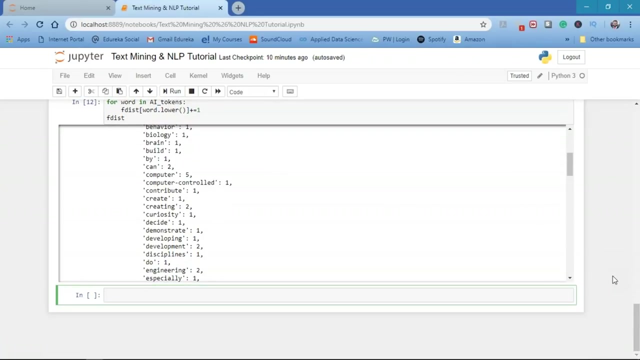 have full stop 9 times and we have accomplished 1, according 1 and so on. We have computer 5 times. Now here we are also converting the tokens into lower case, so as to avoid the probability of considering a word with uppercase and lower case as different. Now suppose we were to select. 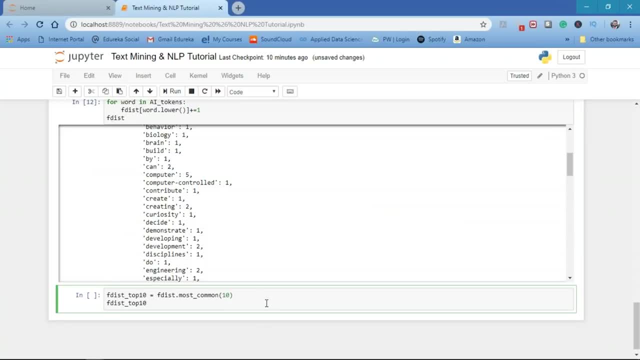 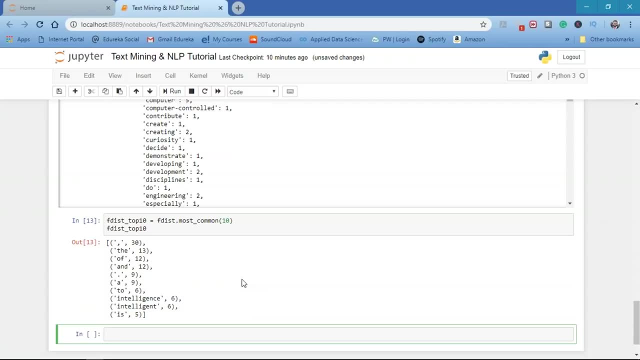 the top 10 tokens with the highest frequency. So here you can see that we have comma 30 times, the 13 times of 12 times and and 12 times, Whereas the meaningful words, which are intelligence, which is 6 times, and intelligence is 6 times. 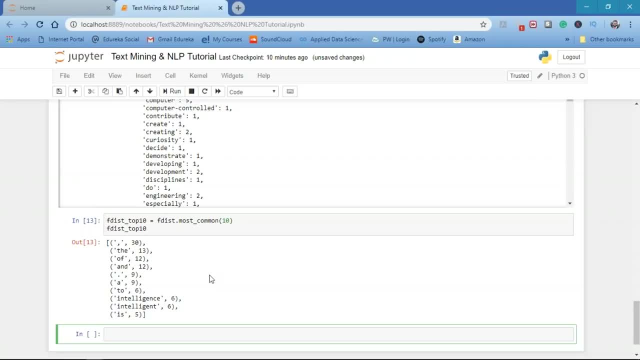 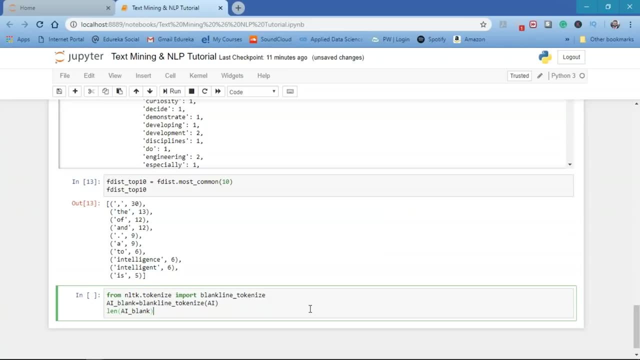 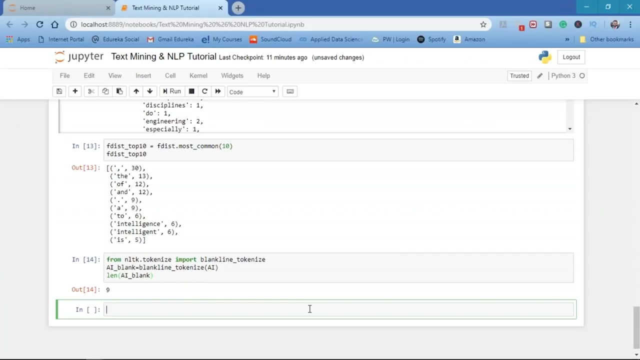 Now there is another type of tokenizer, which is the blank tokenizer. Now let's use the blank tokenizer over the same string to tokenize the paragraph with respect to the blank string. Now the output here is 9.. Now this 9 indicates how many paragraphs we have and what. all paragraphs are separated by a new line. 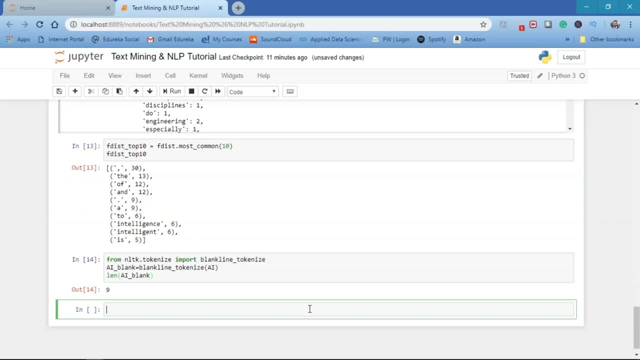 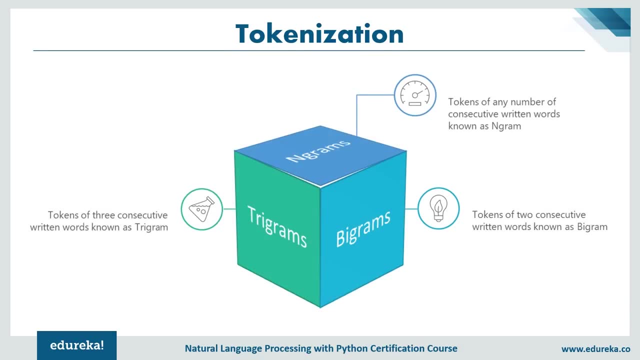 Although it might seem like a one paragraph, it is not. The original structure of the data remains intact. Now, another important key term in tokenizing are bigrams, digrams and ngrams. Now, what does this mean? Now, bigrams refers to tokens of two consecutive words, known as a bigram. Similarly, tokens of three. 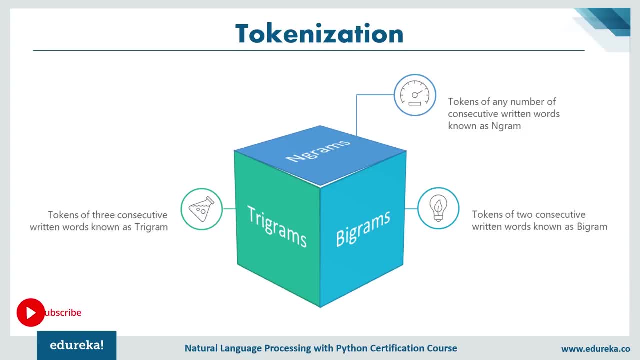 consecutive written words are known as trigram, and similarly we have ngrams for the n consecutive written words. So let's go ahead and execute some demo based on bigrams, digrams and ngrams. So, first of all, what we need to do is 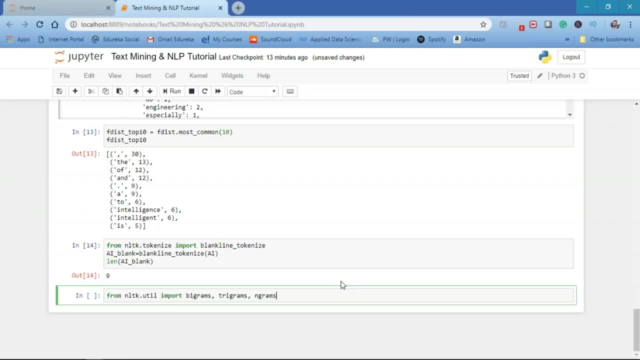 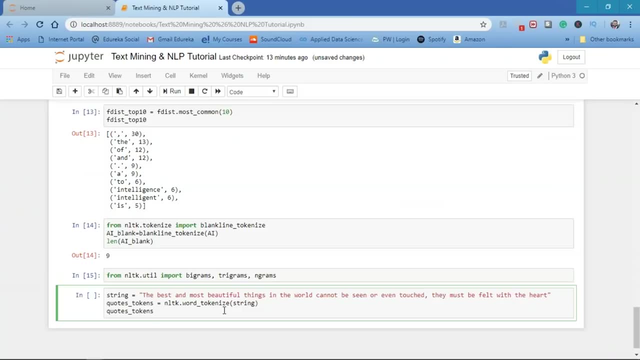 import bigrams, trigrams and ngrams from NLTKutil. Now let's take a string here on which we'll use these functions. So taking this string into consideration. the best and the most beautiful thing in the world cannot be seen or even touched. They must be felt with the heart. So first, what we are. 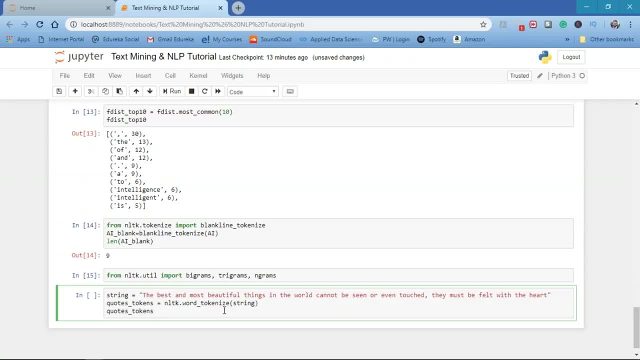 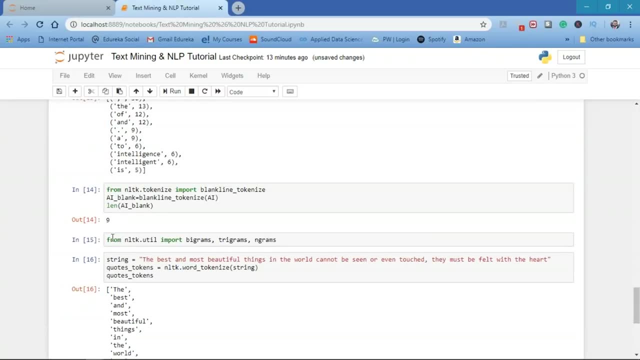 going to do is split the above sentence, or the string, into tokens, So for that we are going to use the word underscore, tokenize. So, as you can see, here we have the tokens Now. let us now create the background of the list containing tokens. 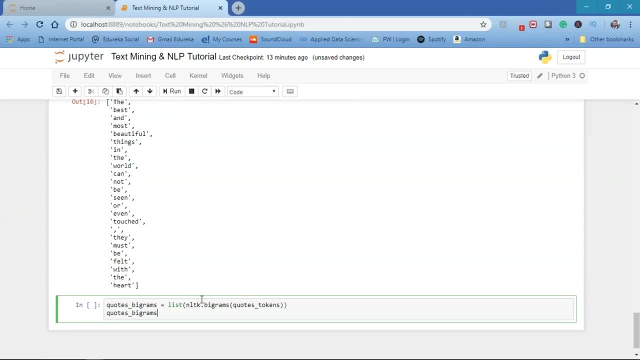 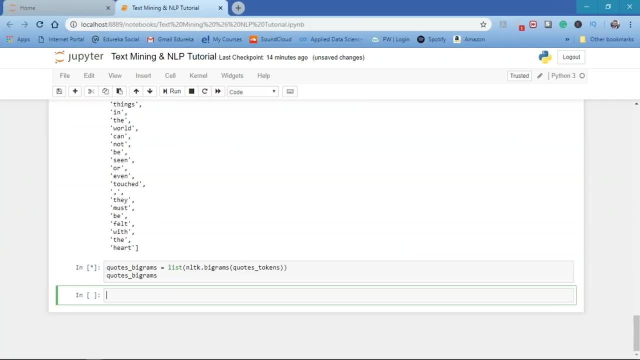 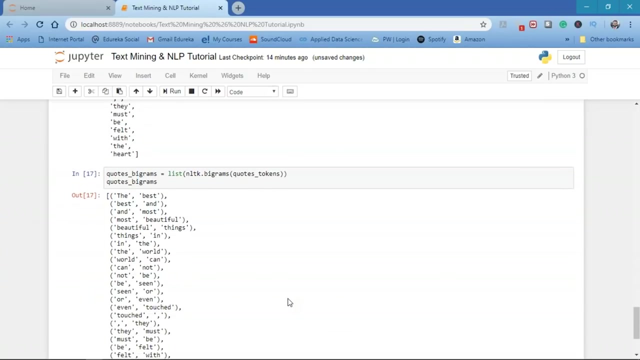 So for that we are going to use the nltk dot bigrams and pass all the tokens And since it is a list, we are going to use the list function. So, as you can see, under output we have the best, best and and most beautiful thing in the world. So, as you can see, the tokens are. 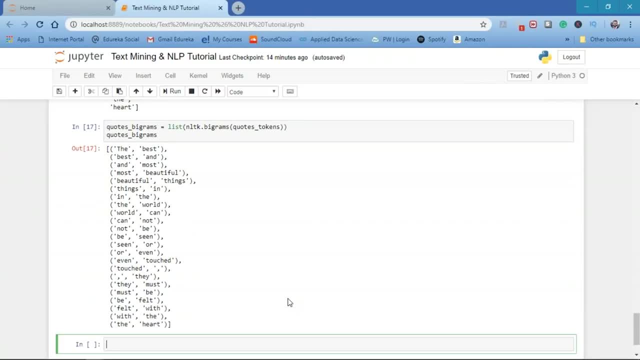 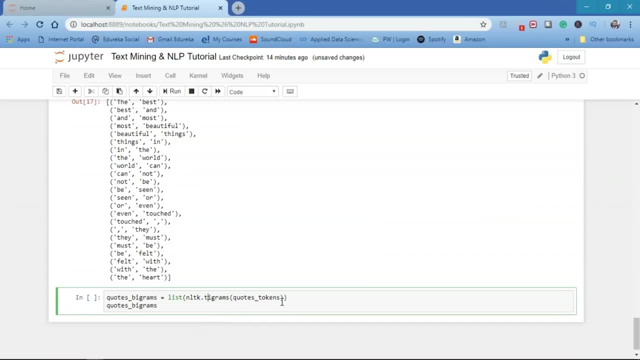 in the form of two words. it's in a pair form. Similarly, if we want to do the trigrams and find out the trigrams, what we need to do is just remove the bigrams and use the trigrams. So, as you can see, we have the. 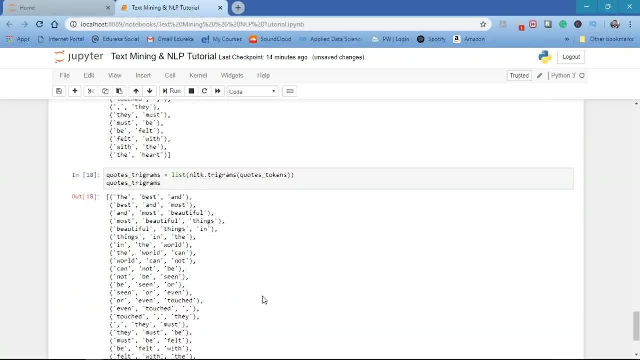 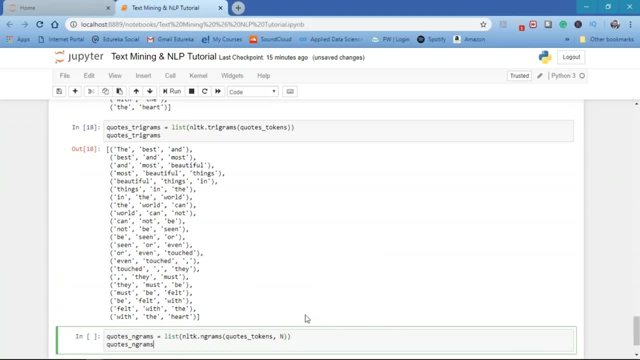 tokens in the form of three words, and if you want to use the n grams, let me show you how it's done. so for n grams, what we need to do is define a particular number here. so, instead of n, i'm going to use, let's say, four. so, as you can see, we have the output in the form of four tokens. 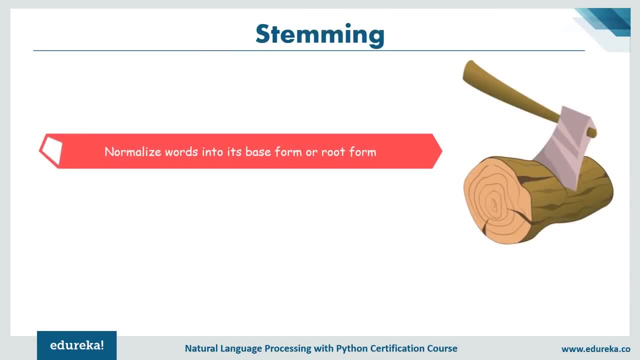 now, once we have the tokens, we need to make some changes to the tokens. so for that we have stemming. now, stemming usually refers to normalizing words into its base form or the root form. so if we have a look at the words here, we have affectation, affects, affections, affected, affection. 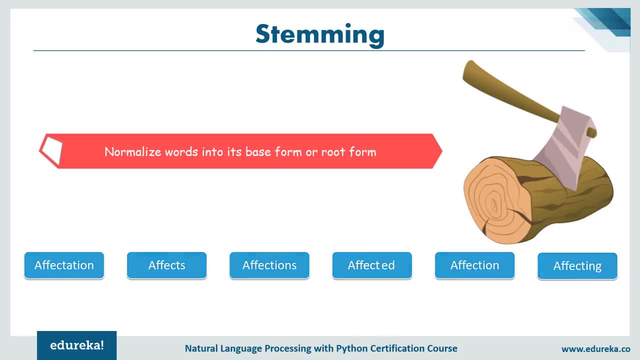 and affecting. so, as you might have guessed, the root word here is affect. so one thing to keep in mind here is that the result may not be the root word always. stemming algorithm works by cutting off the end or the beginning of the word. taking into account a list of common. 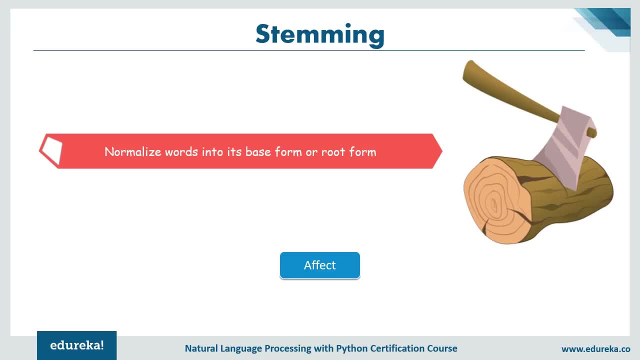 prefixes and suffixes that can be found in an infected world. now, this indiscriminate cutting can be successful in some occasions, but not always, and this is why we affirm that this approach presents some limitations. so let's go ahead and see how we can perform stemming on a particular given data set. now there are quite a few types. 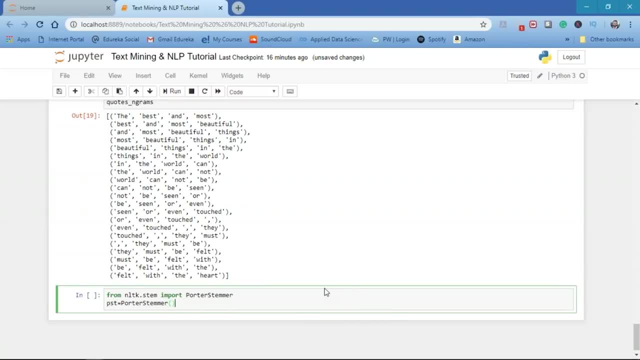 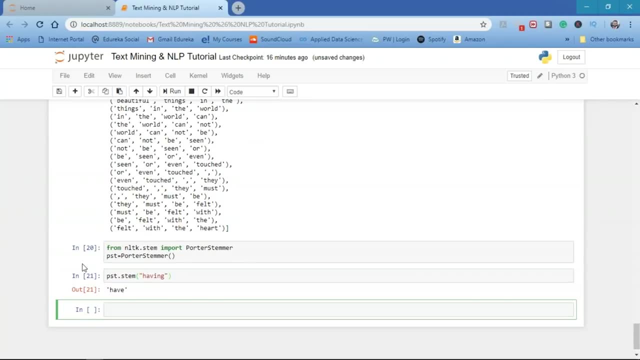 of stem. so, starting with the Potter stem, we need to import it from NLTK dot stem. let's get the output of the word having and see what is the stemming of this word. so, as you can see, we have have as the output. now, here we have defined words to stem which are give, giving, given and gave. so 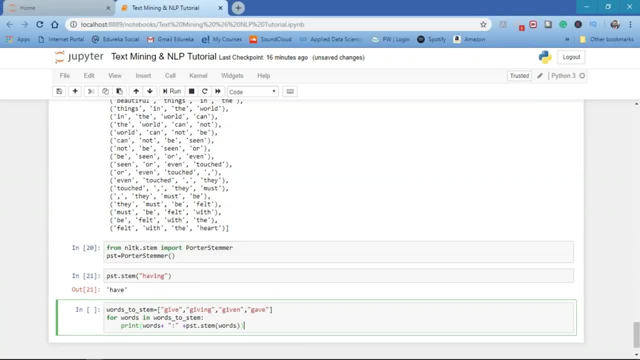 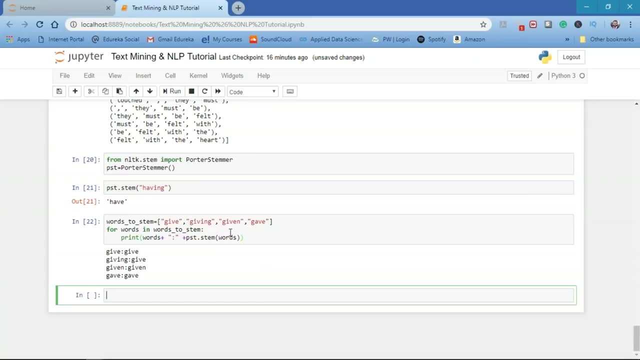 let's use the Potter stemmer and see what is the output of this particular stemming. so you can see it has given, give, given, give and gave. now we can see that the stemmer remove only the ing and replace it with an e. now let's try to do. 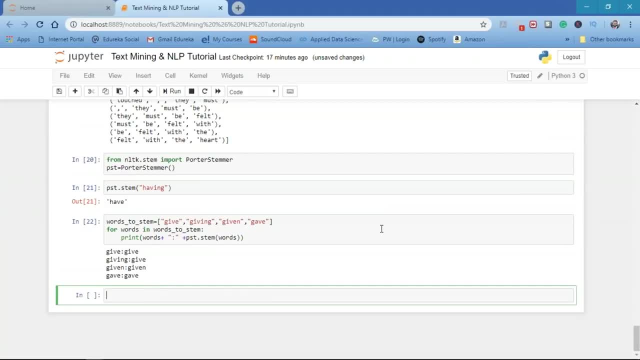 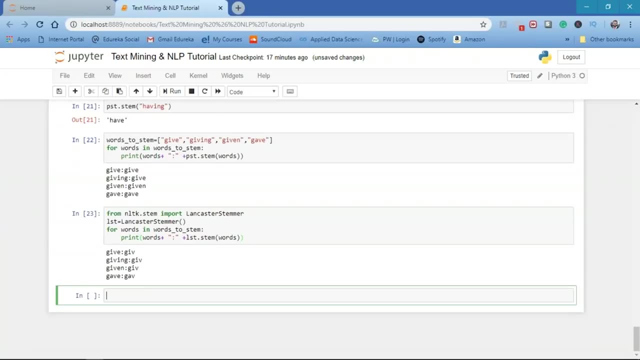 it the same with another stemmer called the Lancaster simmer. you can see the stemmer stem all the words. as a result of it, you can conclude that Lancaster stimmer is more aggressive than the Potter stemmer. not the use of each of these stem applications on the type of tasks that. 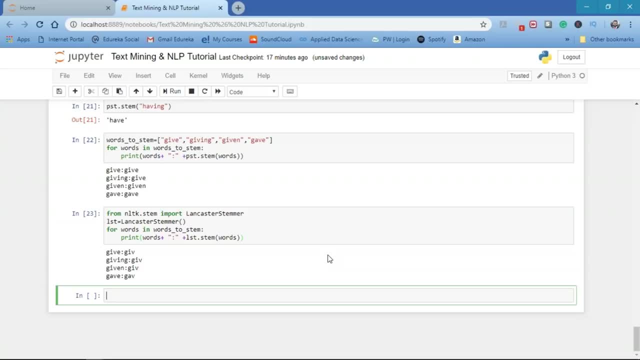 you want to perform. for example, if you want to check how many times the words G, IV is used above, you can use the Lancaster summer and further purposes. you have the Potter simmer as well, but there a lot of spinners. there is one snowball stemmer also present where you need to. 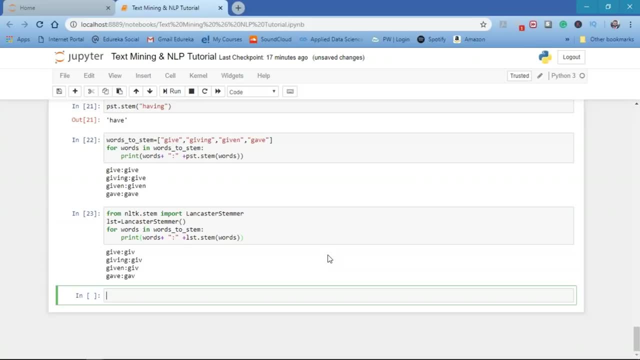 to specify the language which we are using and then use the snowball stemmer. Now, as we discussed, that stemming algorithm works by cutting off the end or the beginning of the word. on the other hand, lemmatization takes into consideration the morphological analysis of the word. 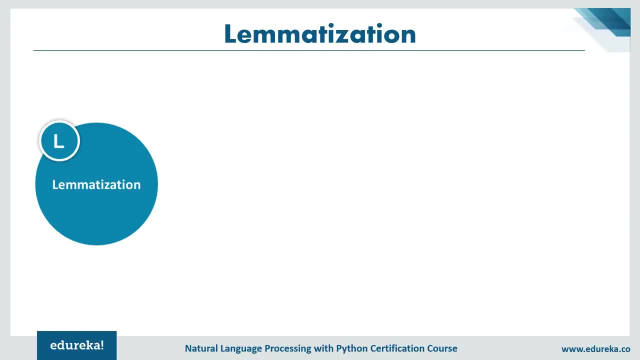 Now, in order to do so, it is necessary to have a detailed dictionary which the algorithm can look into to link the form back to its lemma. Now lemmatization: what it does is groups together different infected forms of a word which are called lemma. it is somehow similar to stemming, as it maps several words into. 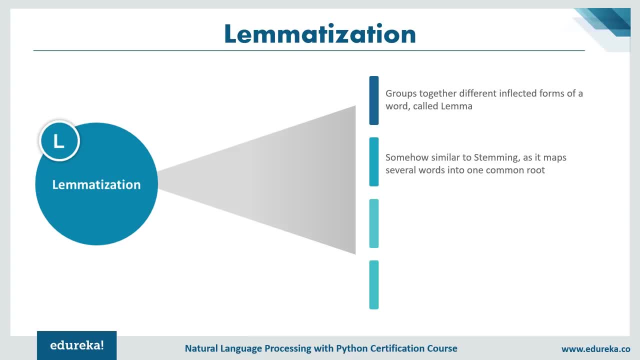 a common root. Now, one of the most important thing here to consider is that the output of lemmatization is a proper word, unlike stemming in that case, where we got the output as giv. now, giv is not any word, it's just a stem. 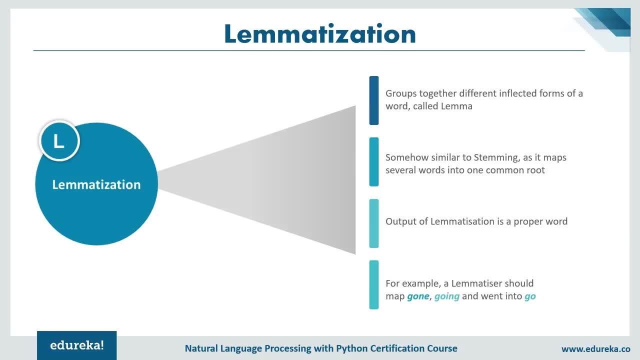 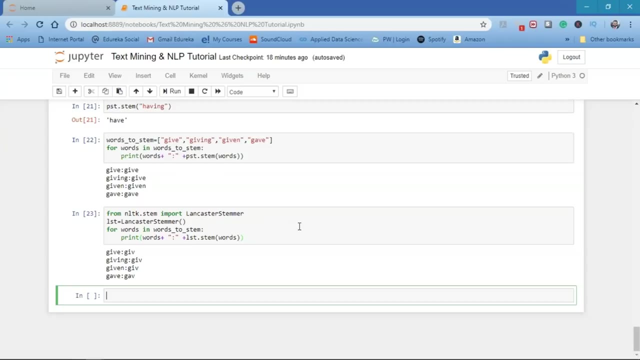 Now, for example, if a lemmatization should work on go on, going and went, It all stems into go, because that is the root of the all the three words here. So let's go ahead and see how lemmatization work on the given input data. 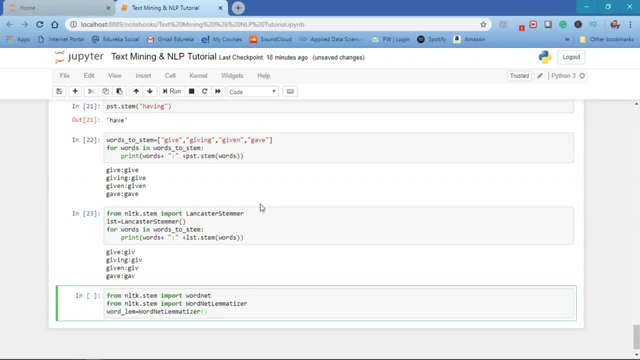 Now for that. we are going to import the lemmatizer from NLTK. Now we are also importing the word net here, As I mentioned earlier that lemmatization requires a detailed dictionary because the output of it is a root word, which is a particular given word. it's not just any random word. it. 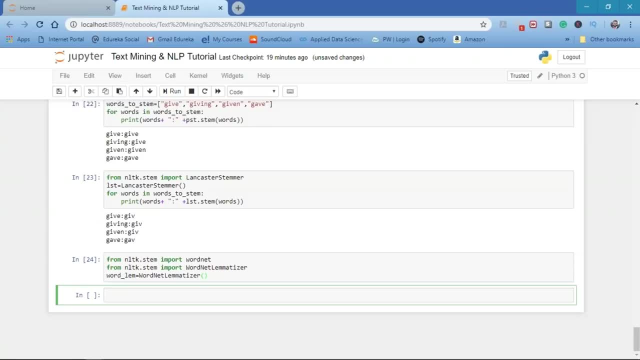 is a proper word. So to find that proper word it needs a dictionary. So here we are providing the word net dictionary and we are using the word that lemmatizer, So passing the word corpora into the word net lemmatizer. 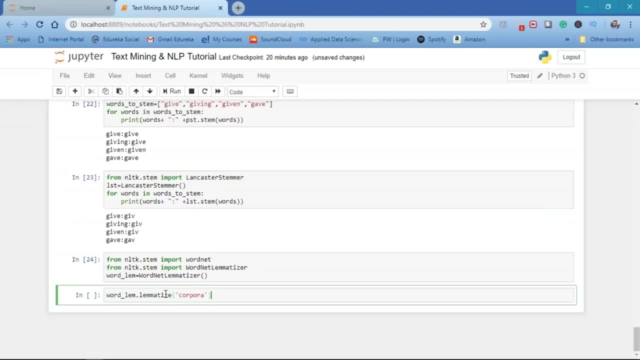 So can you guys tell me what is the output of this one? I'll leave this up to you guys. I won't execute the sentence. Let me remove the sentence here. You guys tell me in the comments below what will be the output of the lemmatization of: 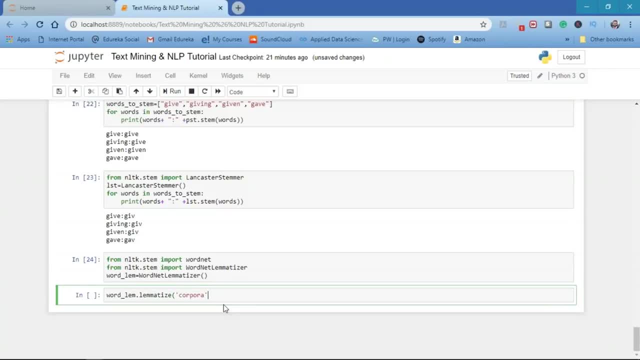 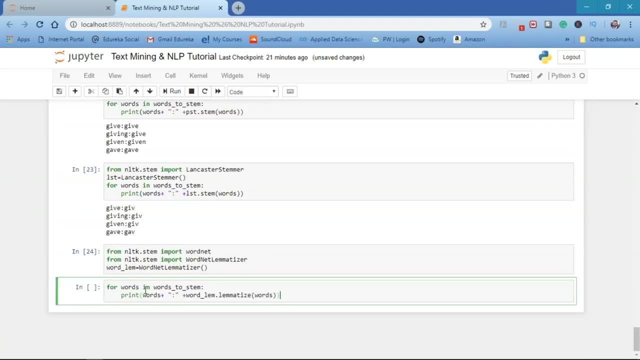 the word corpora and what really the output of the stemming? you guys execute that and let me know. Let me know in the comments section below. Now let's take these words into consideration: give, giving, given and gave and see what is the output of the lemmatization. 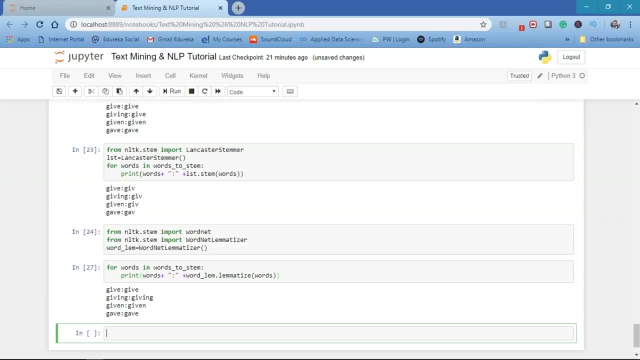 So, as you can see here, the lemmatizer has kept the words as it is, and this is because we haven't assigned any POS tags here, and hence it has assumed all the words as nouns. Now you might be wondering: what are POS tags? 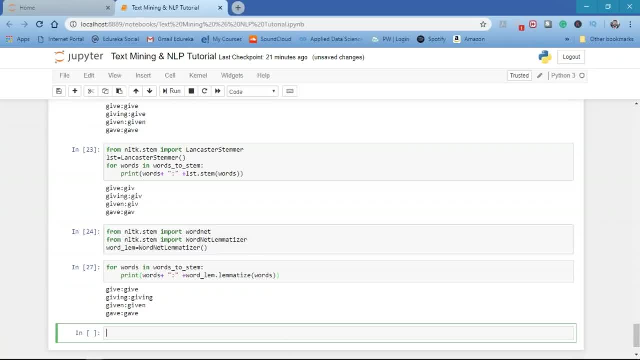 Well, I'll tell you what are POS tags later in this video. So for just now, let's keep it as simple as that. Is that? POS tags usually tell us what exactly the given word is. Is it a noun, Is it a verb or is it different parts of speech? 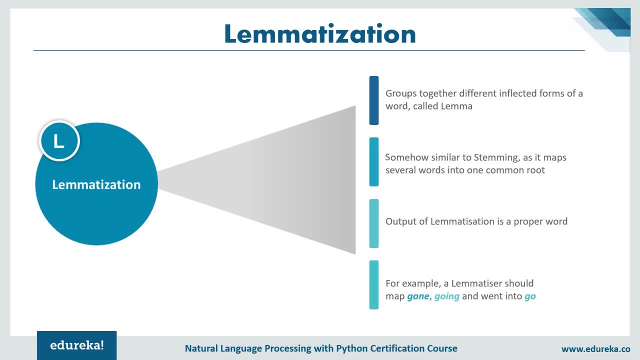 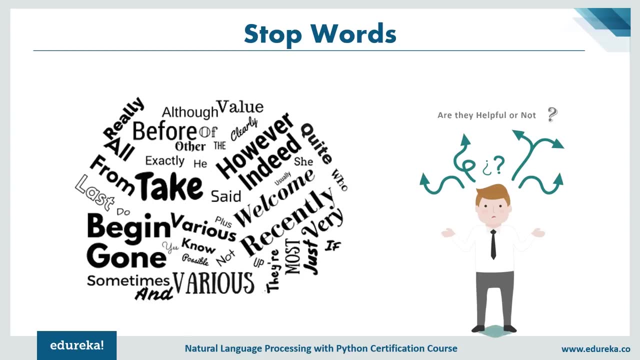 Basically, POS stands for parts of speech. Now, do you know that there are several words in the English language, such as I ate for above below, which are very useful in the formation of sentence and without it the sentence would make any sense. But these words do not provide any help in the natural language processing. and this list 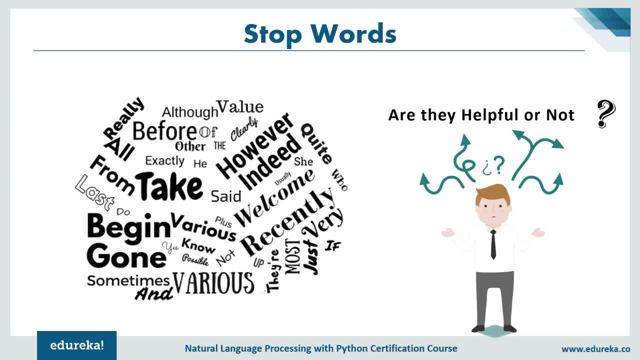 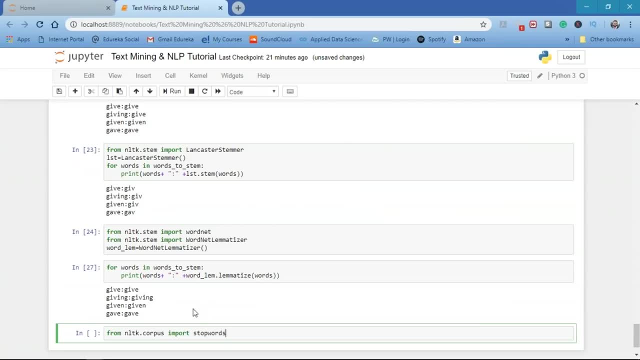 of words, Also known as stop words, and LTK has its own list of stop words and you can use the same by importing it from the NLTK dot corpus. So the question arises: are they helpful or not? Yes, they are helpful in the creation of sentences, but they are not helpful in the processing. 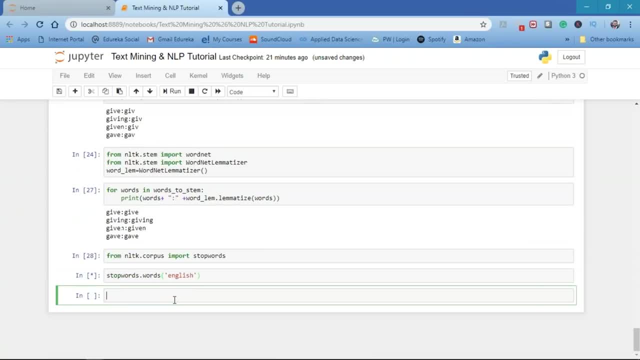 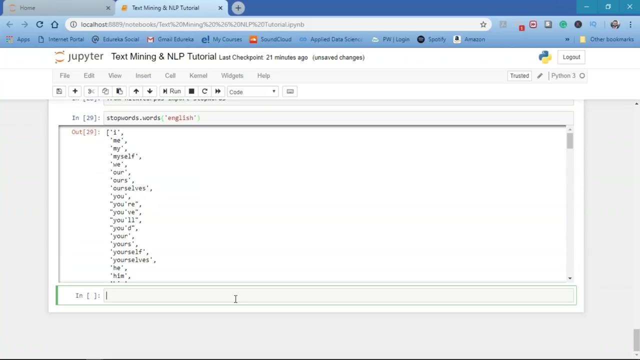 of the language. So let's check the list of stop word in the NLTK. So from NLTK dot corpus we are importing the stop words and if we specify what all stop words are there in the English language, Let's see. So you can see here we have the list of all the stop words which are defined in the English. 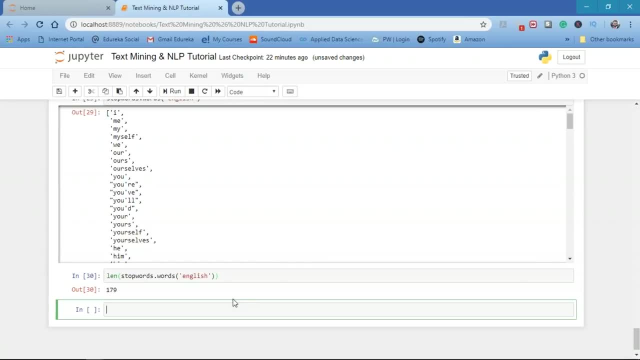 language and we have one hundred and seventy nine total number of stop words. Now, as you can see, here we have these words, which are few more, most others. Now, these words are very necessary in the formation of sentences. You cannot ignore these words, but for processing these are not important at all. 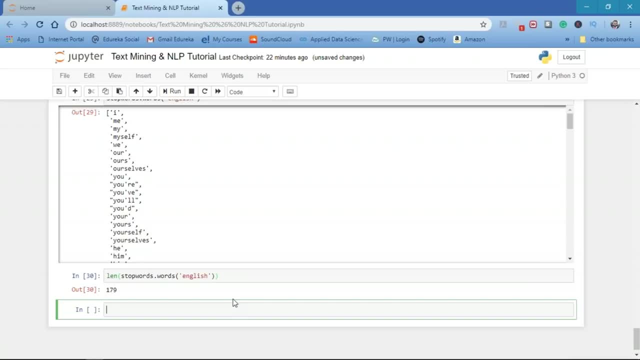 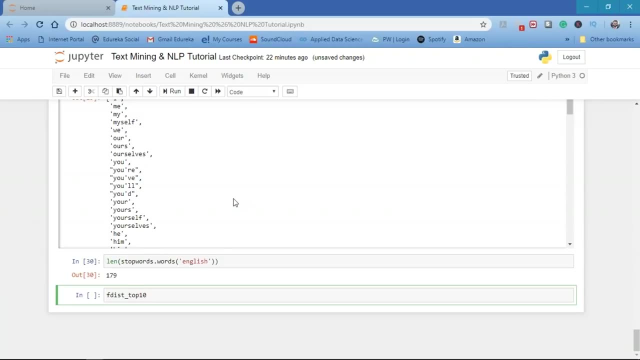 So, if you remember, we had the top 10 tokens from that particular Word, that is, the AI paragraph I mentioned earlier, which was given as F test underscore top 10.. Let's take that into consideration and see what you can see here. is that except intelligent? 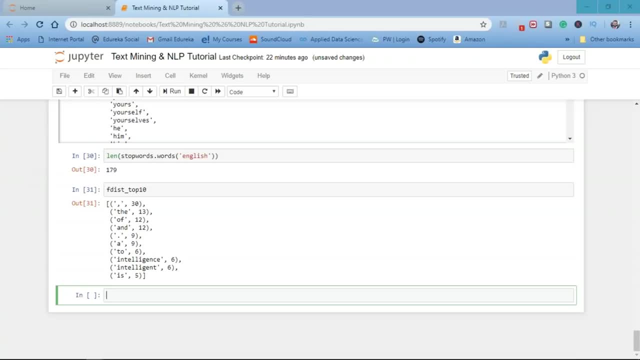 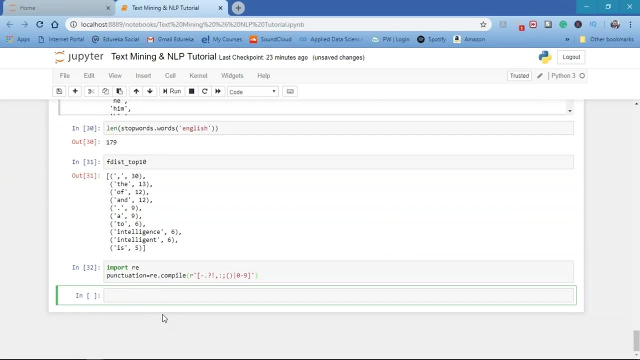 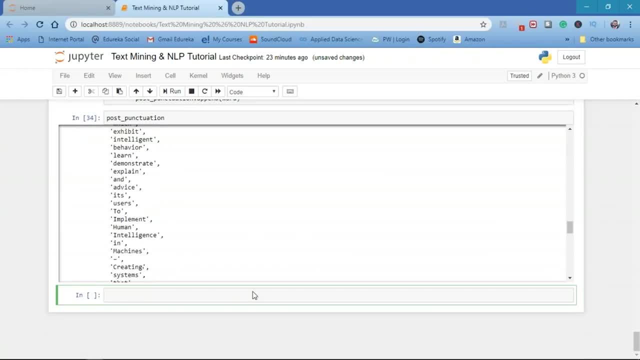 So if we have a look at the output of the post punctuation, So if we have a look at the output of the post punctuation, So if we have a look at the output of the post punctuation, You can see there are no stop words here in the particular given output. 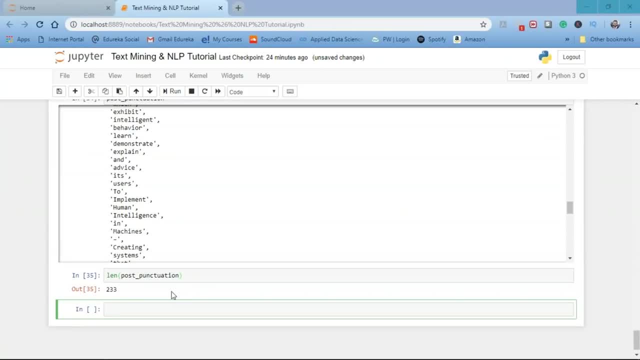 And if you have a look at the output of the length of the post punctuation, it's 233 compared to the 273, the length of the AI underscore tokens. Now, this is very necessary in language processing, as it removes the all the unnecessary words which do not hold any much more meaning. 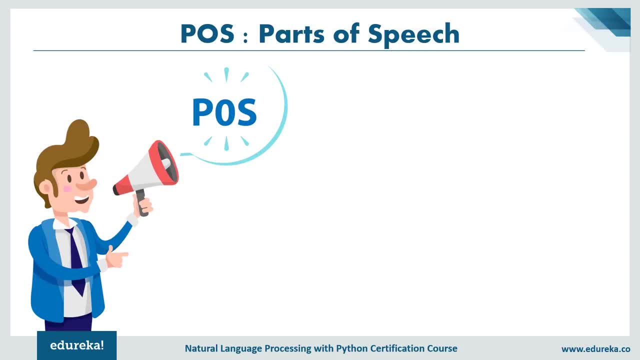 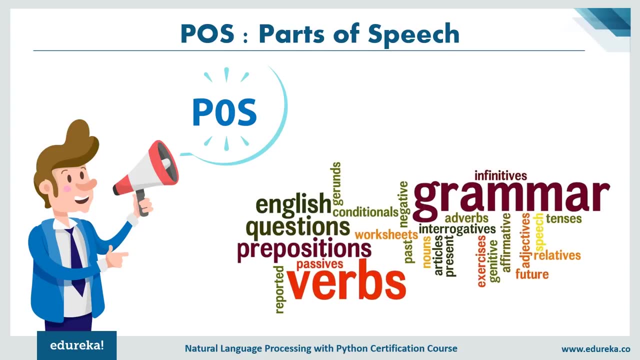 Now coming to another important topic of natural language processing and text mining, or text analysis, is the parts of speech. Now, generally speaking, the grammatical type of the word, which is the verb, noun adjective adverb article, indicates how a word functions in the meaning as well as the grammatical. 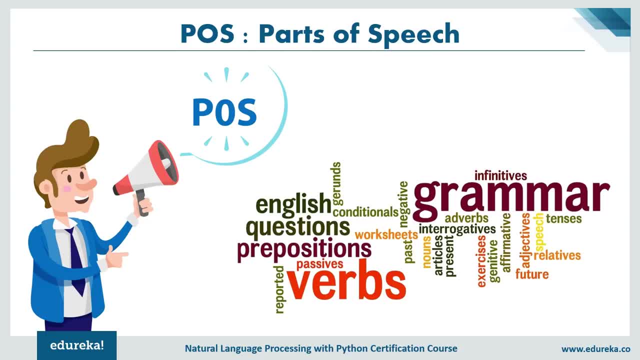 within the sentence. Now, a word can have more than one parts of speech based on the context in which it is used. For example, if you take that sentence into consideration, Google something on the Internet. Now, here Google acts as a verb, although it is a proper noun. 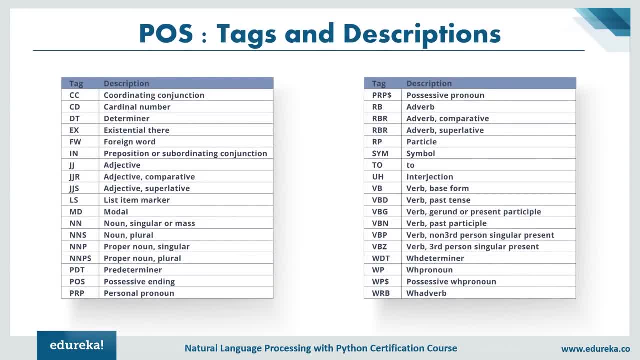 So, as you can see, here We have so many types of POS tags and we have the descriptions of those various tags. So we have the coordinating conjunction CC, cardinal number CD. We have JJ as adjective, MD as modal, We have the proper noun singular plural. 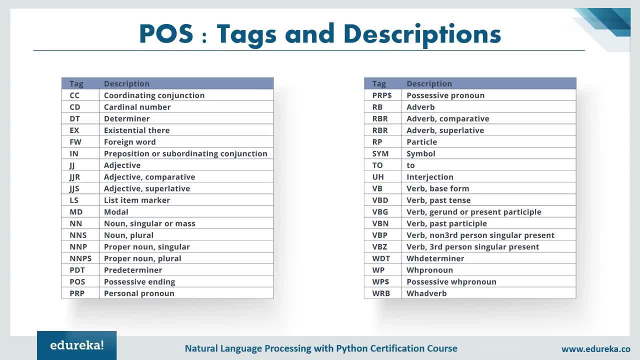 We have verbs, different types of words, We have interjection symbol, We have the Y pronoun and the Y adverb. Now we can use POS tags as a statistical NLP task. It distinguishes the sense of the word, which is very helpful in text realization and it 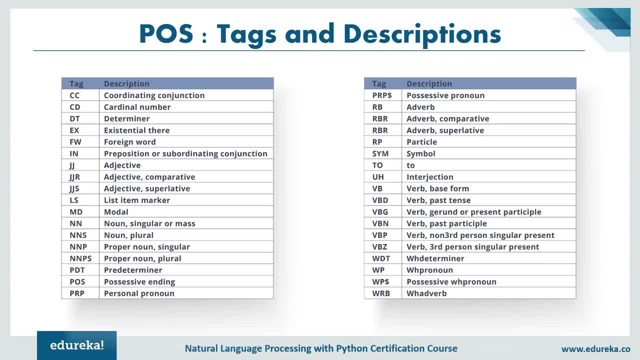 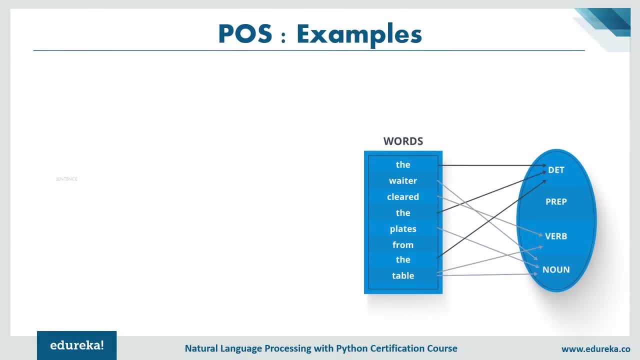 is easy to evaluate, as in how many tags are correct, and you can also infer semantic information from the given text. So let's have a look at some of the examples of POS. So take the sentence the dog killed the bat. So here the is a determiner, dog is a noun, killed is a verb and again the bat are determiner. 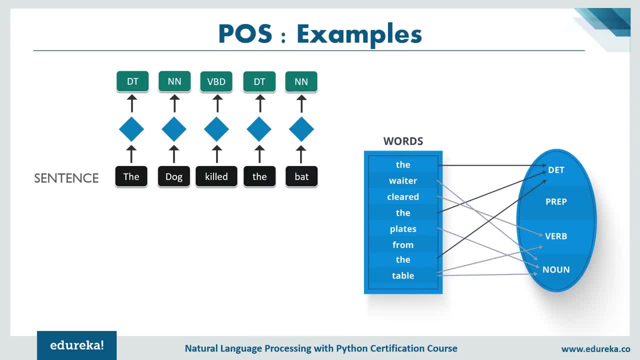 and noun respectively. Now let's consider another sentence: the way to clear the plates from the table. So, as you can see here, all the tokens here correspond to a particular type of tag, which is the parts of speech tag. It is very helpful in text realization. 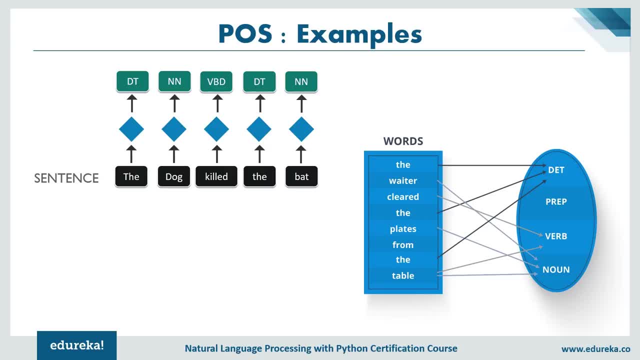 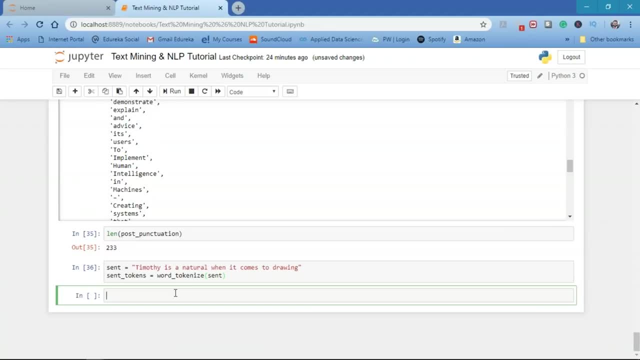 Now let's consider a string and check how NLTK performs POS tagging on it. So let's take the sentence: Timothy is a natural when it comes to drawing. first we are going to tokenize it and under NLTK only, we have the POS underscore tag option and will pass. 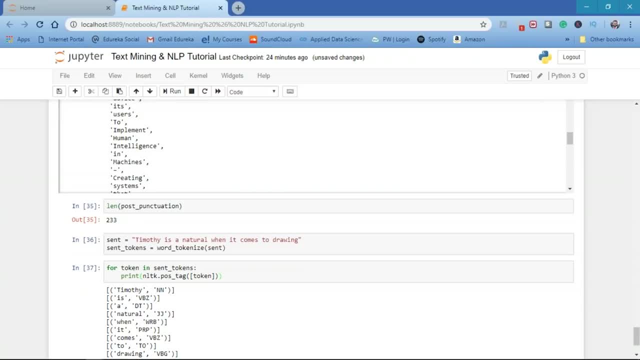 all the tokens here. So as you can see, we have Timothy as noun is a verb or as a determiner natural, as an adjective, when, as a verb it, as a preposition, comes as a verb to, as a to, and drawing as a verb again. 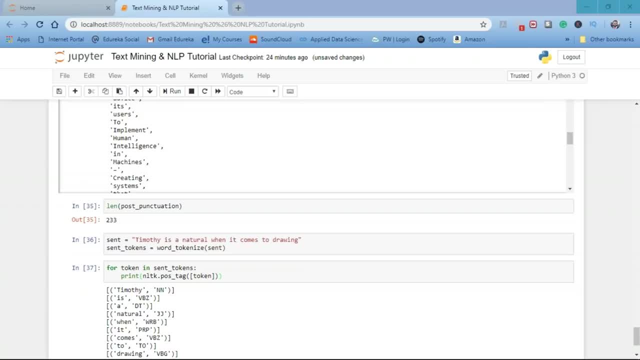 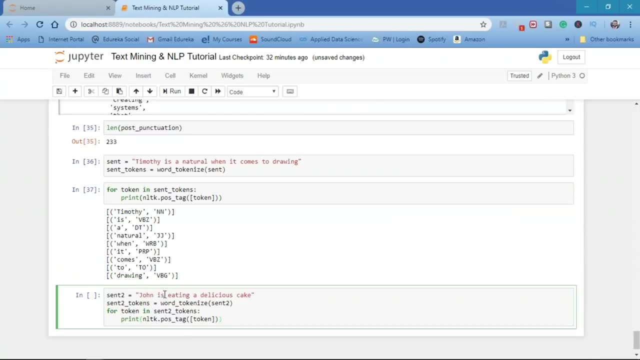 So this is how you define the POS tags. The POS underscore tag function does all the work here. Let's take another example. here, John is eating a delicious cake. Let's see what's the output of this one. Now, here you can see that the tagger has. 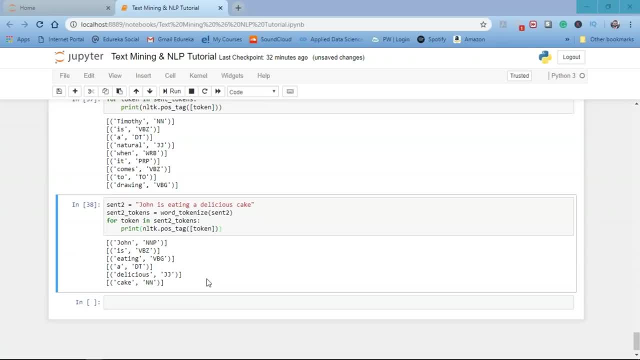 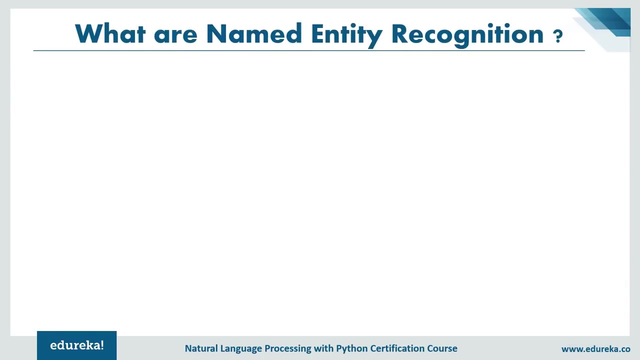 Tag both the word is and eating as a verb, because it has consider is eating as a single term. This is one of the few shortcomings of the POS taggers, One thing important to keep in mind. Now, after POS tagging, there is another important topic, which is the named entity recognition. 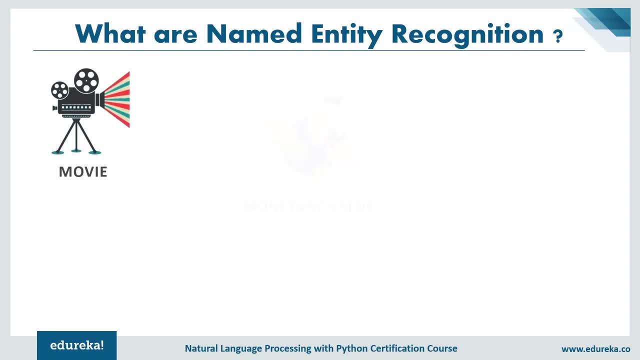 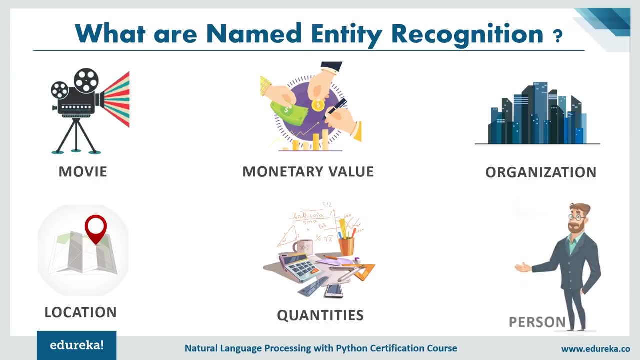 So what does it mean? Now, the process of detecting the named entities, such as the person name, the location name, the company name, the organization, the quantities and the monitoring, The value, is called the name, entity recognition. Now, I don't name entity recognition. We have three types of identification here. 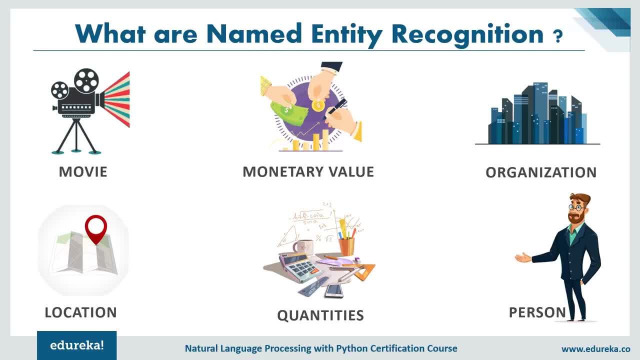 We have the non phase identification, Now this step, these with the extracting all the noun phrases from a text using dependency, passing and parts of speech tagging. Then we have the phrase classification, the step classification. This is the classification step in which all the extracted noun phrases are classified. 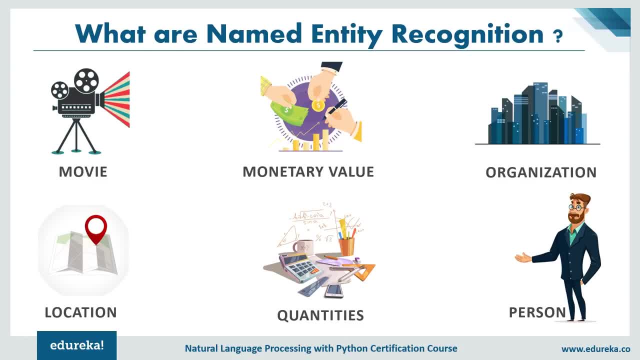 into respective categories, which are the location names, Organization and much more. and apart from this, one can curate the lookup tables and dictionaries by combining information from different sources. And finally, we have the entity disambiguation. Now, sometimes it is possible that the entities are misclassified. 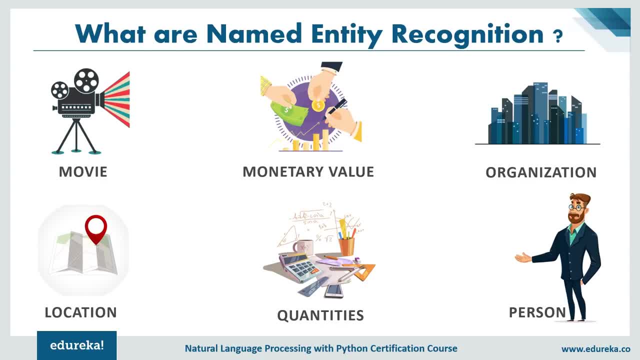 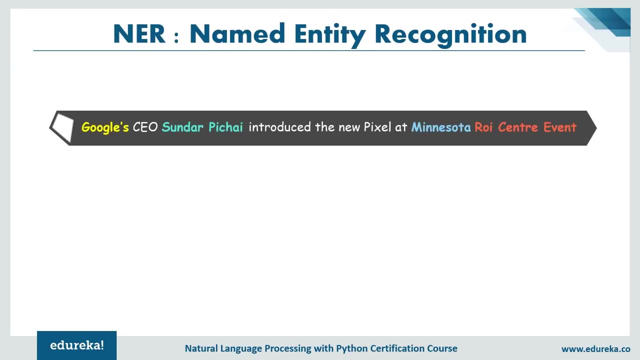 Hence, creating a validation layer on top of the result is very useful, and the use of knowledge graphs can be exploited for this purpose. Now, the popular knowledge graphs are Google knowledge graph, the IBM Watson and Wikipedia. So let's take a sentence into consideration That the Google CEO, Sundar Pichai, introduced a new pixel at Minnesota Roy Center event. 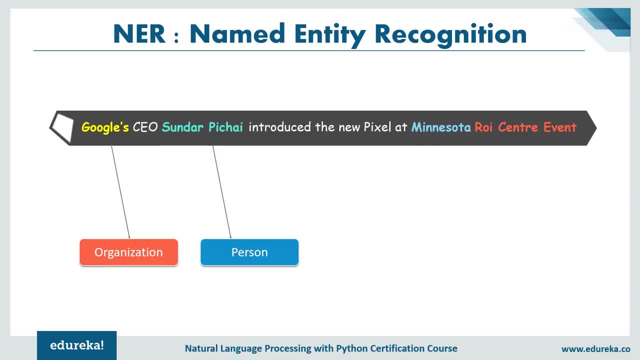 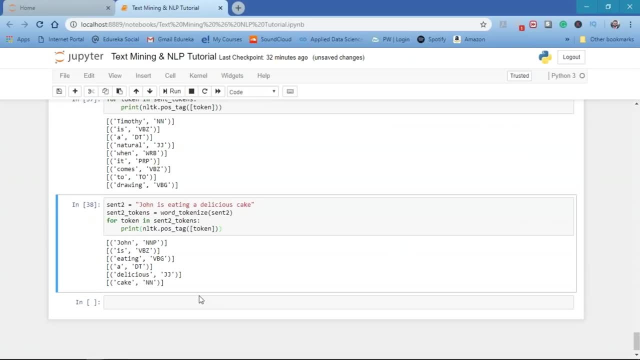 So, as you can see here, Google is an organization, Sundar Pichai as a person, Minnesota as a location and the Roy Center event is also tagged as an organization For using NER in Python will have to import the NEE underscore chunk from the NLTK module. 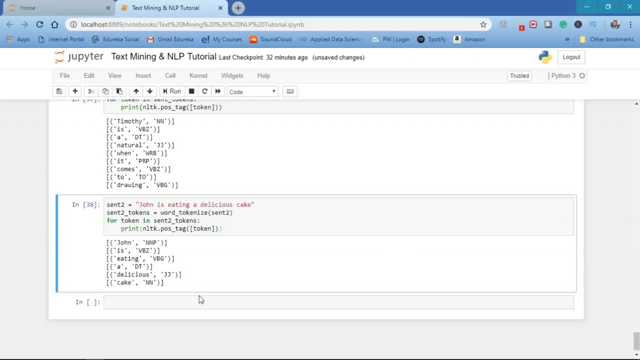 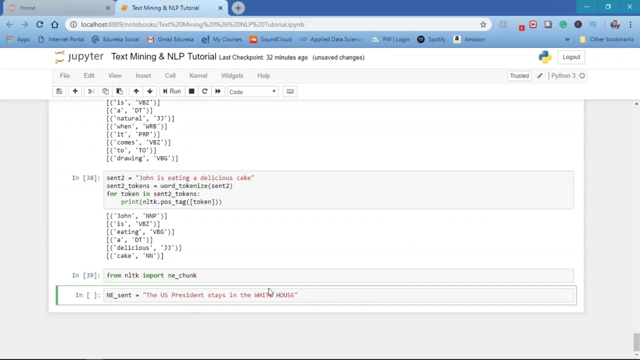 which is present in Python. So let's consider our text data here and see how we can perform the NER using the NLTK library. So first we need to import the NEE underscore chunk here. Let's consider the sentence here We have: the US president stays in the White House. 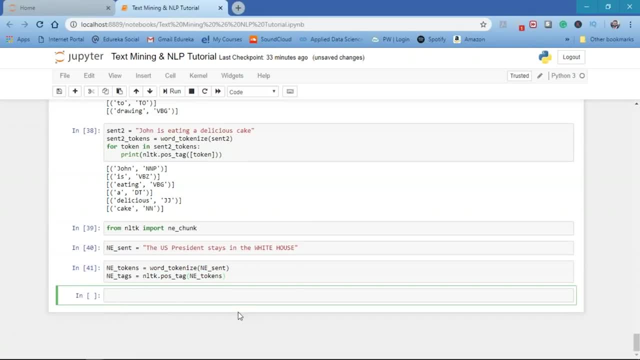 So we need to do all these processes again. We need to tokenize the sentence first and then add the POS tags, and then, if we use the NEE underscore chunk function and pass the list of tuples containing POS tags to it, Let's see the output. 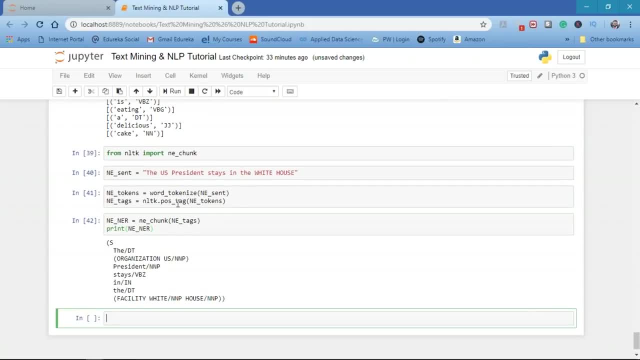 So, as you can see, the US here is recognized as an organization And White House is clubbed together as a single entity and is recognized as a facility. Now, this is only possible because of the POS tagging. without the POS tagging, it would be very hard to detect the named entities of the given tokens. 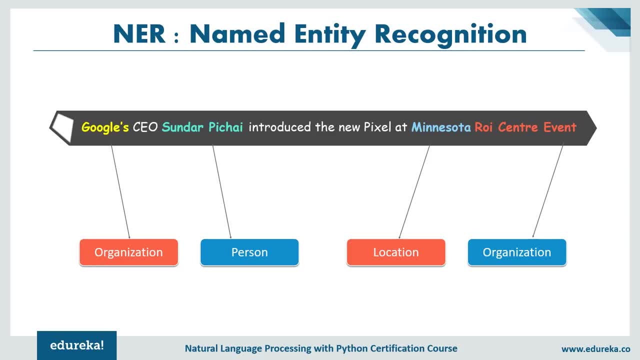 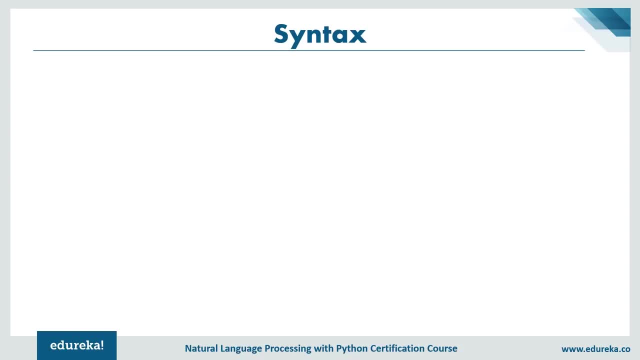 Now that we have understood what are named entity recognition and NERs, Let's go ahead and understand one of the most important topic in NLP and text mining, which is the syntax. So what is the syntax? So, in linguistics, syntax is the set of rules, principles and the processes that govern the 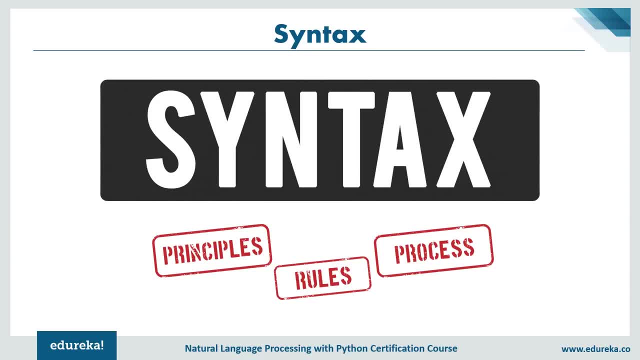 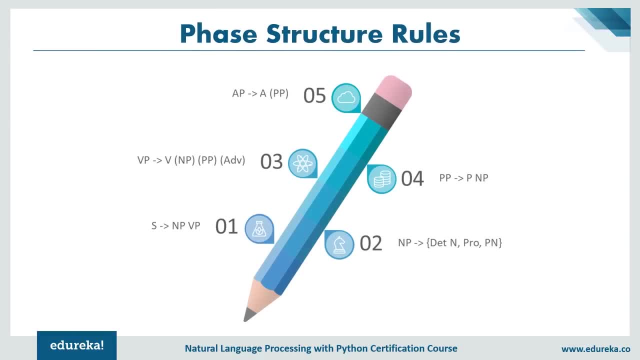 structure of a given sentence in a given language. The term syntax is also used to refer to the study of such principles and processes. So what we have here are certain rules as to what part of the sentence should come at what position. with these rules, one can create a syntax tree whenever there is a sentence. 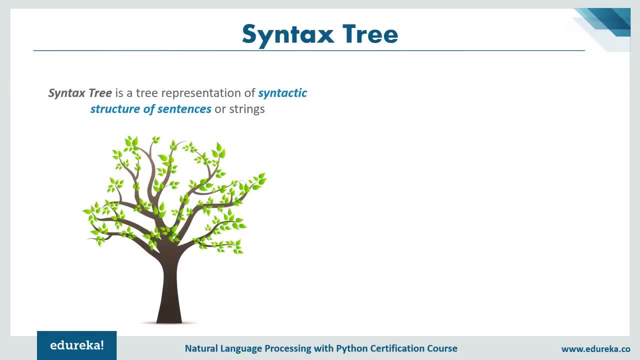 input Now. syntax tree, in layman terms, is basically a tree representation of the syntactic structure of the sentence, of the strings. It is a way of representing the syntax of a programming language as a hierarchical tree structure. This structure is used for generating symbols, tables for compilers and later code generation. 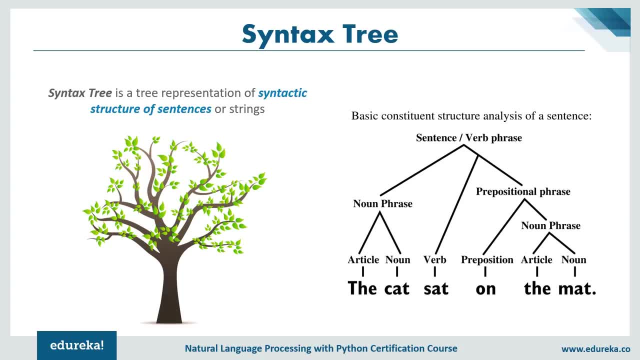 The tree represents all the constructs in the language and their subsequent rules. So let's consider the statement. the cat sat on the mat. So, as you can see, here the input is a sentence or a verb phrase And it has been classified into non-phrase and the prepositional phase, again the noun. 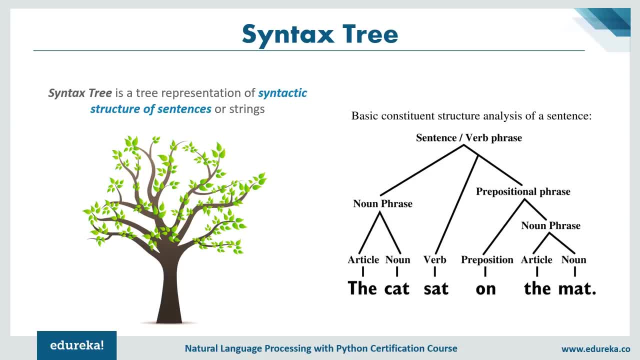 phrase is classified into article and noun, and again we have the verb, which is sat, and finally we have the preposition on the article and the noun, which are the and Matt. now, in order to render syntax trees in our notebook, You need to install the ghost strip, which is a rendering engine. 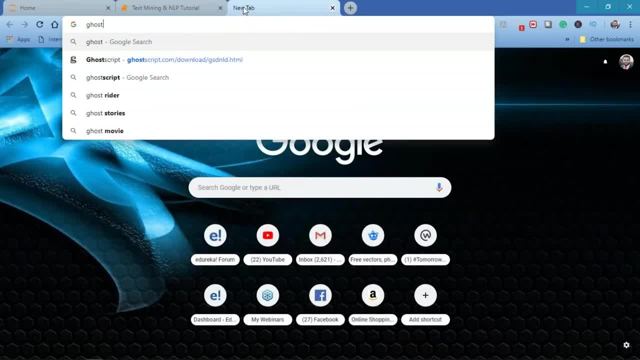 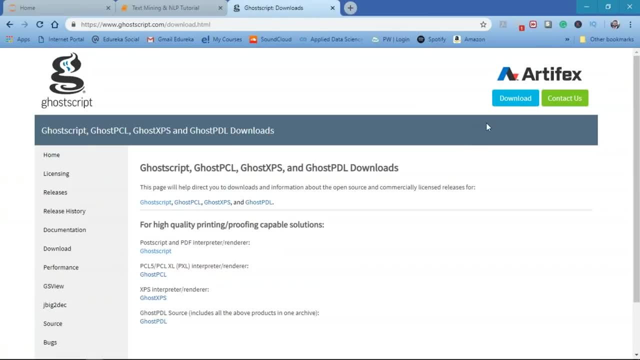 Now this takes a lot of time, and let me show you from where you can download the course script. Just type in download Go script And select the latest version here. So, as you can see, we have two types of license here. We have the general public license and the commercial license as creating syntax and 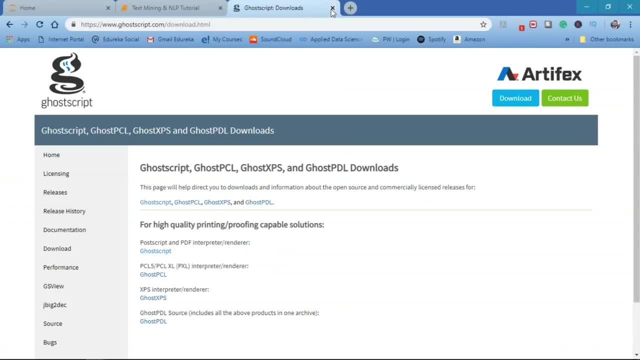 following. it is a very important part. It is also available for commercial license and it is very useful. So I'm not going to go much deeper into what syntax tree is and how we can do that. So now that we have understood what are syntax trees, 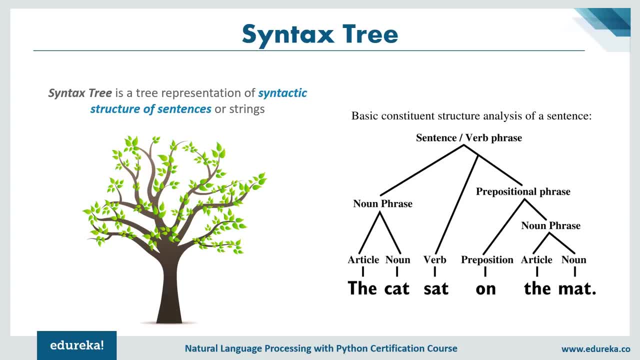 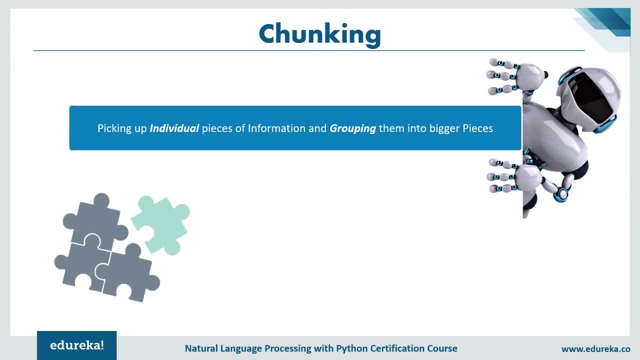 Let's discuss The concept with respect to analyzing the sentence structure, which is chunking. So chunking basically means picking up individual pieces of information and grouping them into bigger pieces, And these bigger pieces are also known as chunks in the context of NLP and text mining. 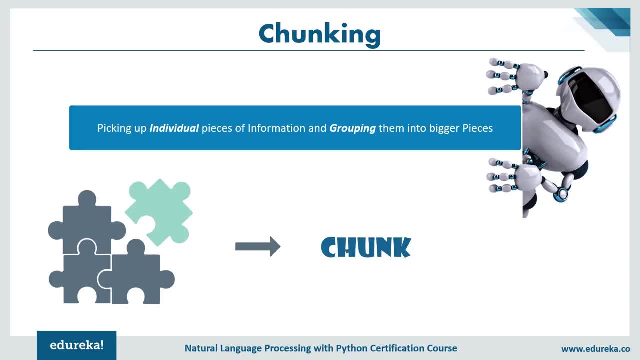 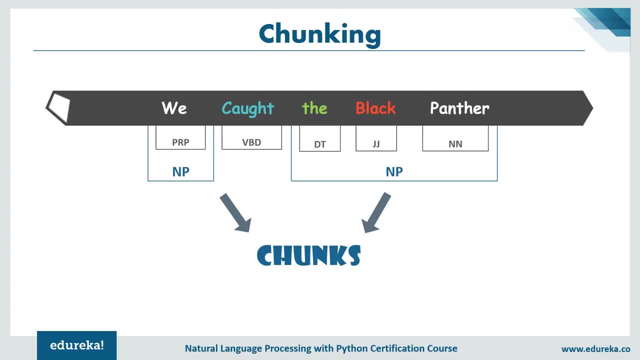 chunking means grouping of words or tokens into chunks. So let's have a look at the example here. So the sentence into consideration here is: we caught the Black Panther V is the preposition caught The determiner. black is an adjective and Panther is a noun. 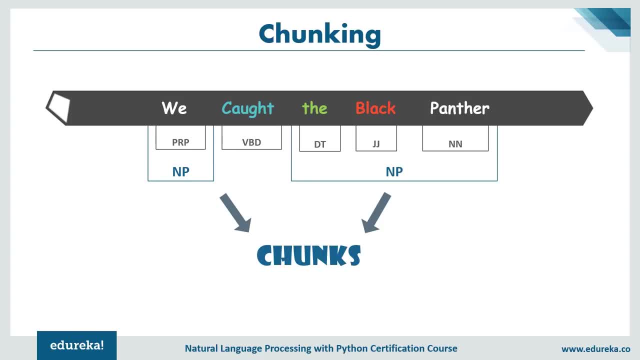 So what it has done is here, as you can see, is that pink, which is an adjective, Panther, which is a noun, and D is a determiner, are chunked together in the noun phrase. So let's go ahead and see how we can implement chunking using the NLTK. 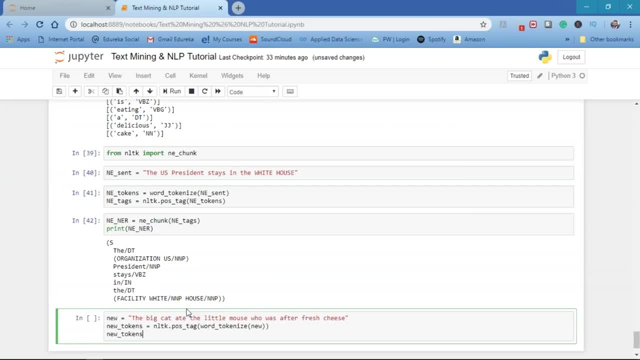 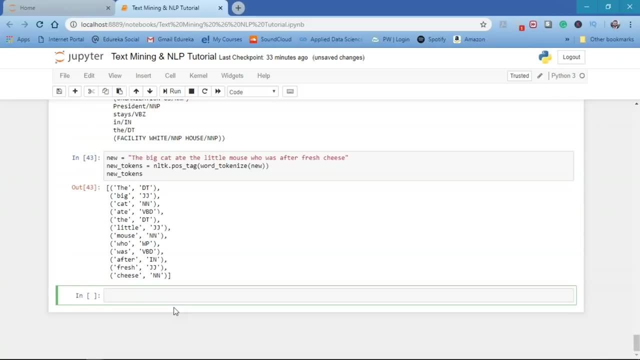 So let's take the sentence: the big cat ate little mouse who was after the fresh cheese. We'll use the POS tags here and also use the tokenizing function here. So, as you can see, here we have the tokens and we have the POS tags. 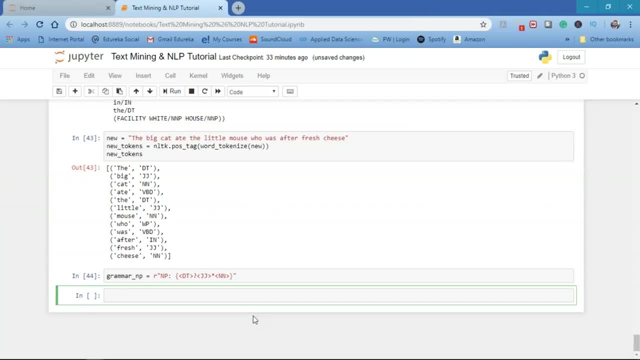 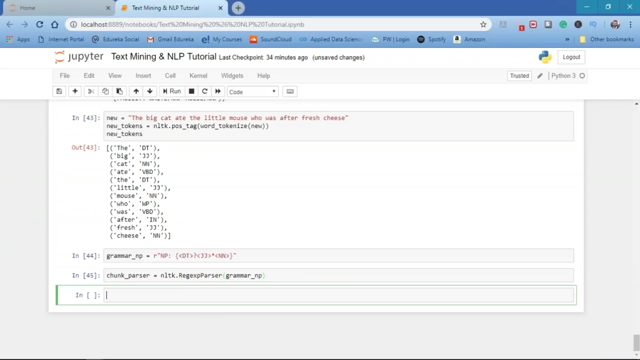 What we'll do now is create a grammar from a noun phrase and will mention the tags that we want in our chunk phrase within the curly braces. So that will be our grammar underscore: NP. Now here we have created a regular expression matching string. Now we'll now have to pass the chunk and hence will create a chunk pass and pass our non. 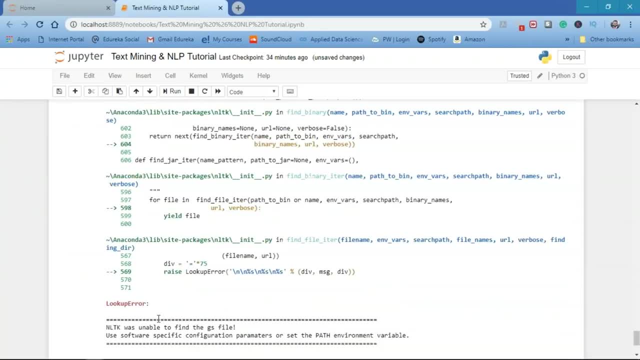 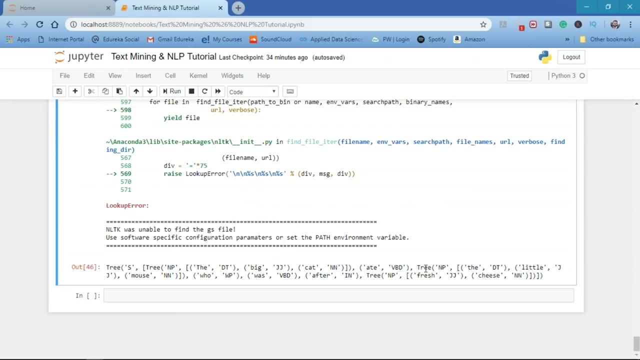 free string to it. So, as you can see, We have a certain error and let me tell you why this error occurred. So this error occurred because we did not use the code script and we do not form the syntactical tree, But in the final output we have a tree tree structure here which is not exactly in the 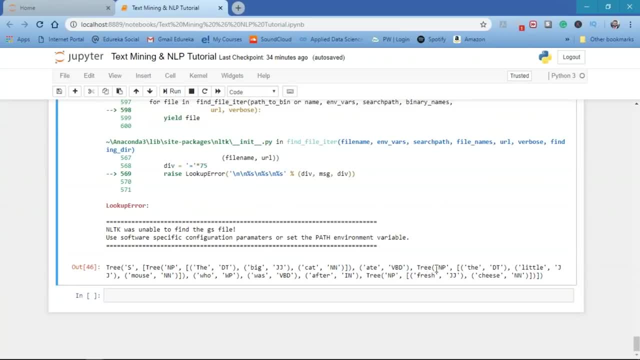 visualization part, but it's there. So, as you can see, here we have the NP noun phrase for the little mouse. again We have the noun phrase for fresh cheese also. All the fresh is an adjective, Cheese is a noun. It has considered a noun phrase of these two words. 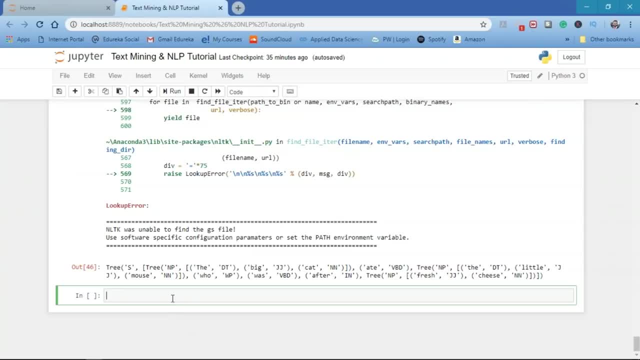 So this is how you execute chunking in NLTK library. So by now we have learned almost all the important steps in text processing and let's apply them all in building a machine learning classifier on the movie reviews from the NLTK corpora. So for that, first let me import all the libraries, which are the Pandas, the NumPy library, 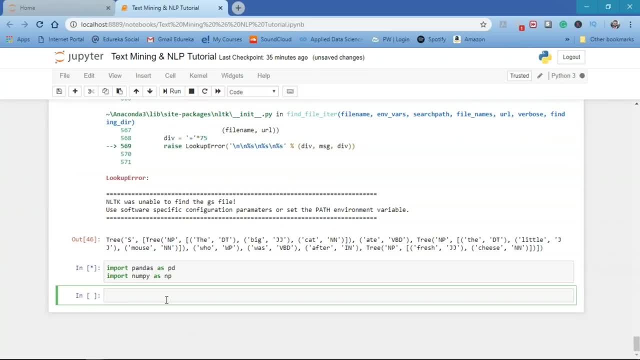 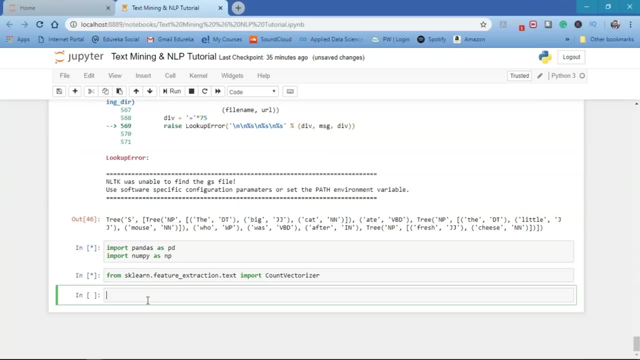 Now, these are the basic libraries needed in any machine learning algorithm. We are also importing the count vectorizer. I'll tell you why it is used later. now Let's just import it for now. So again, if we have a look at the different elements of the corpora, as we saw earlier, 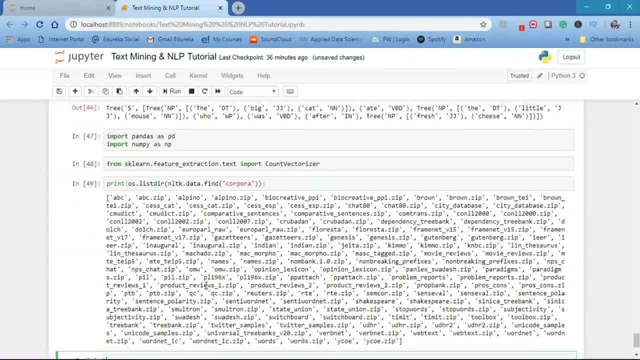 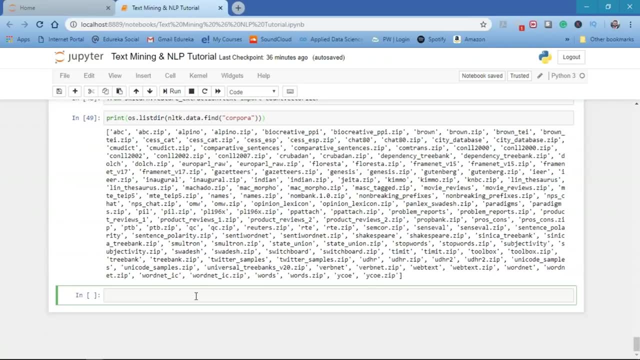 in the beginning of our session. we have so many files in the given NLTK corpora. Let's now access the movie reviews corporas under the NLTK corpora. As you can see, here we have the movie reviews for that. We are going to import the movie underscore reviews from the NLTK corpora. 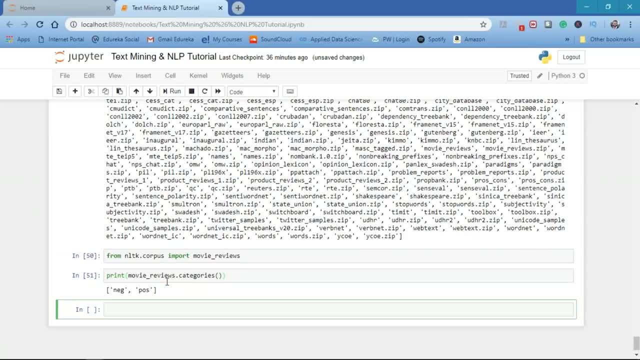 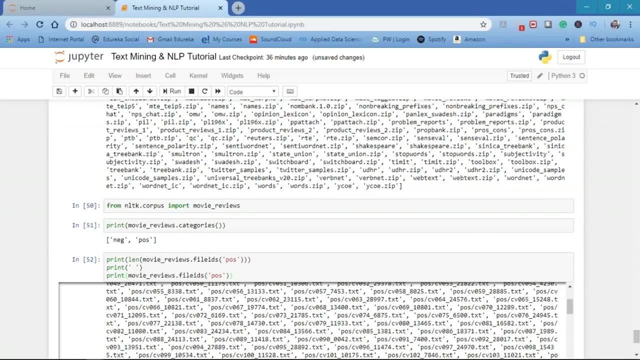 So let's import the movie reviews from the movie underscore reviews from the NLTK corpora. So if we have a look at the different categories of the movie reviews, we have two categories which are the negative and the positive. So if you have a look at the positive, we can see we have so many text files here. 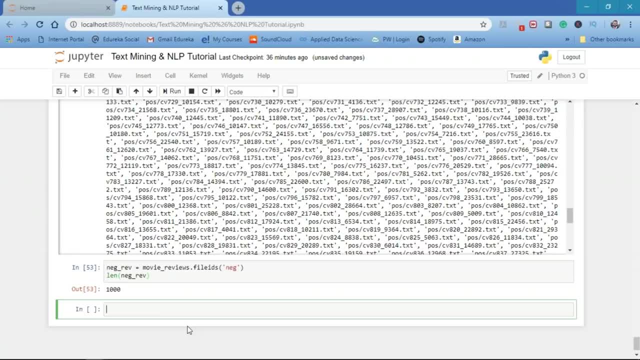 Similarly, if we have a look at the negative, we have thousand negative files also here which have the negative feedbacks. So let's take a particular positive one into consideration, which is the CV double zero, two, nine, five, nine zero. You can take any one of the files here. 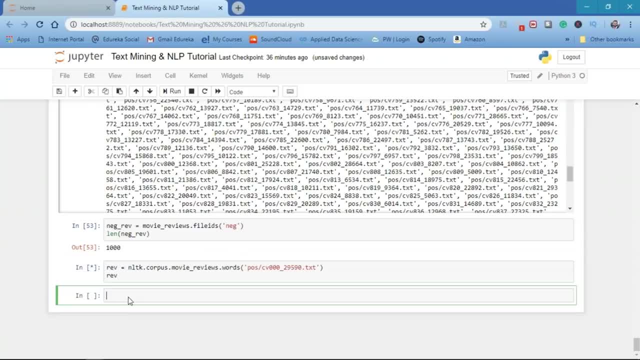 It doesn't matter Now the above tokenization. as you can see here the file is already tokenized, but it is generally useful for us to do the tokenization. But the above tokenization has increased our work here and in order to use the count vectorizer. 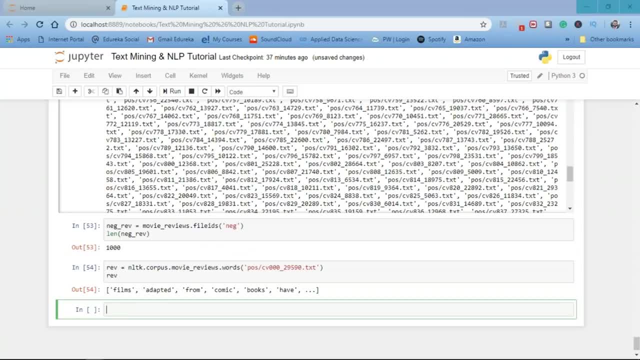 and the TF idea. we must pass the strings instead of the tokens. Now, in order to convert the strings into token, we can use the D tokenizer within the NLTK, but that has some licensing issues as of now with the with the conda environment. 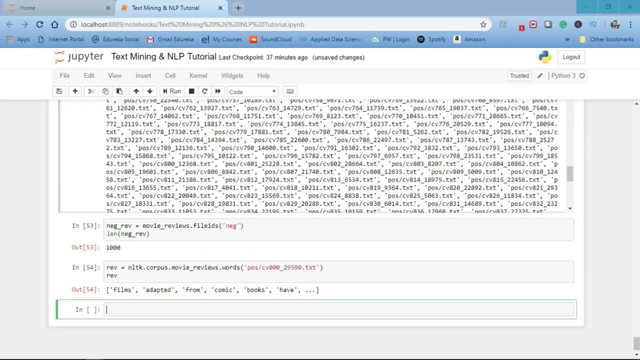 So instead of that, we can also use the join method to join all the tokens of the list into a single string, and that's what we are going to use here. So first we are going to create an empty list and append all the tokens within it. 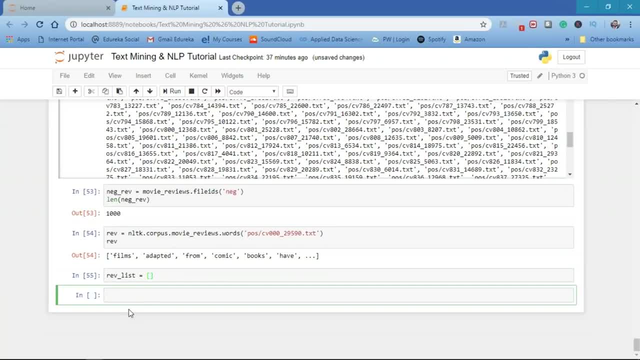 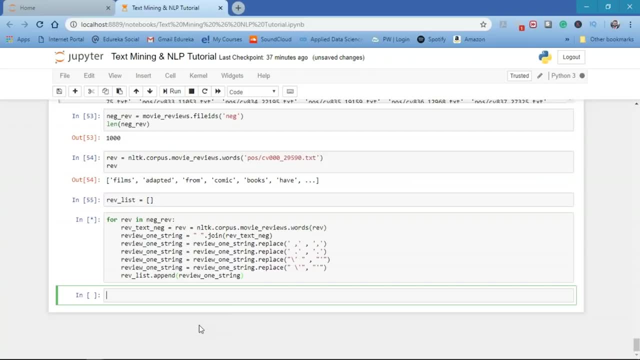 We have the review underscore list. that is an empty list. Now, what we are going to do here is remove all the extra spaces, the commas, from the list while appending it to the empty list, and perform the same For the positive and the negative reviews. 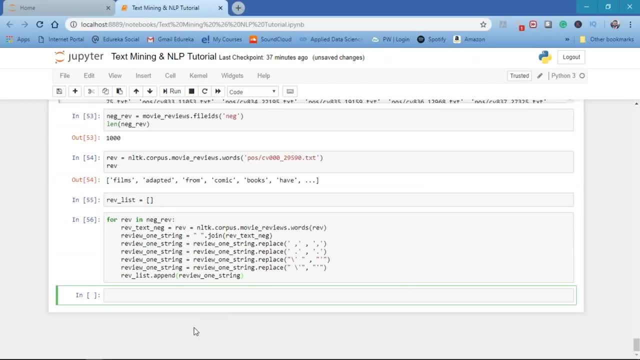 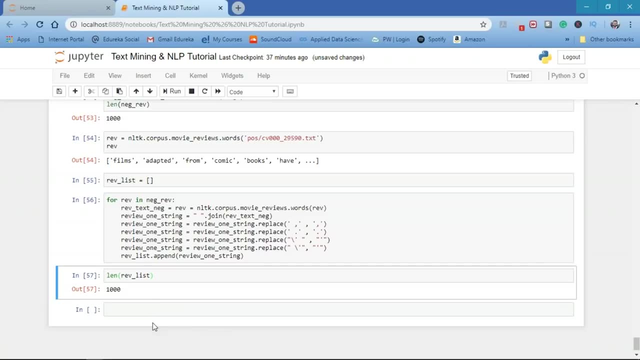 So this one, we are doing it for the negative reviews and then we'll do the same for the positive reviews as well. So if you have a look at the length of this negative review list, it's thousand, and the moment we add the positive reviews. 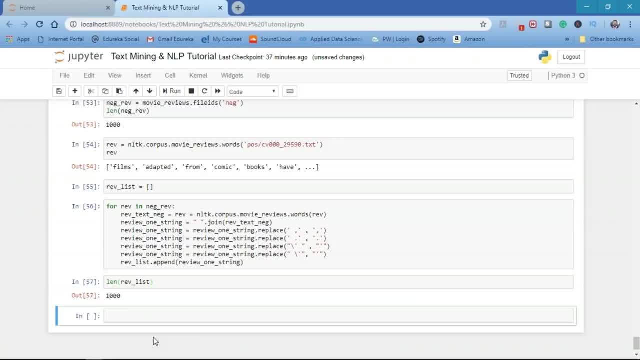 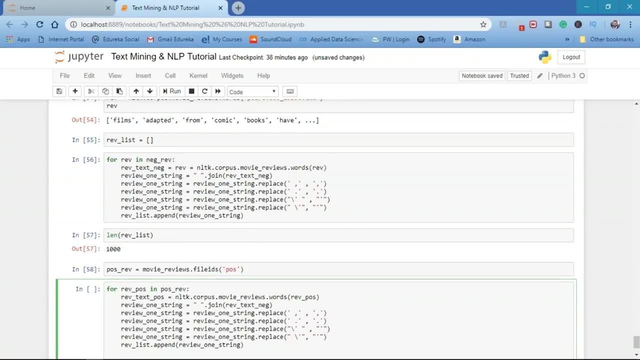 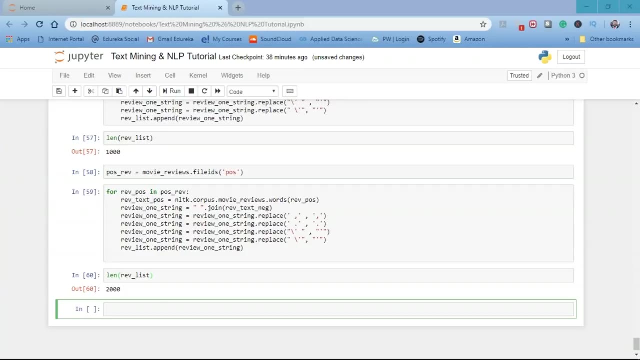 Also, I think the land should reach 2000.. So let me just Define the positive reviews, Now execute the same for positive reviews And then again, if we have a look at the length of the review list, it should be 2000. that is good. 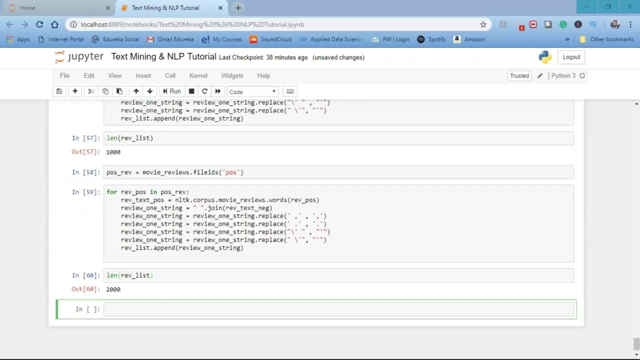 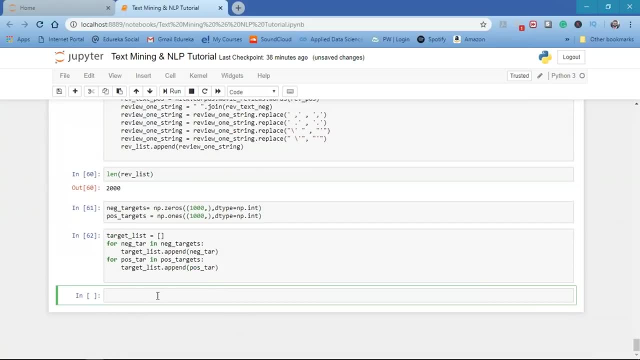 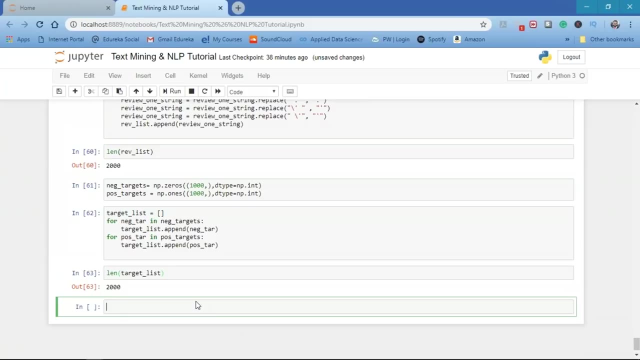 Now, let us now create the targets before creating the few features for our classifiers. So, while creating the targets, we are using the negative reviews- here We are denoting it as zero, and for the positive reviews, We are converting it into one, and also we will create an empty list. 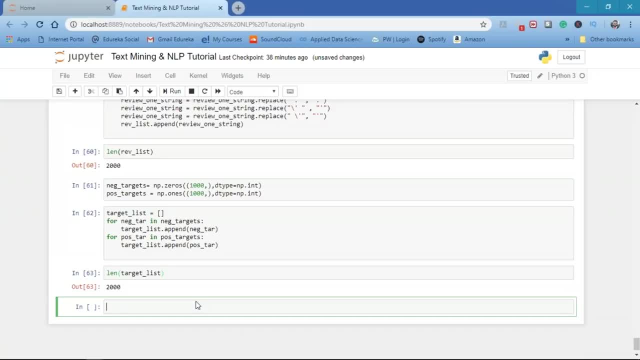 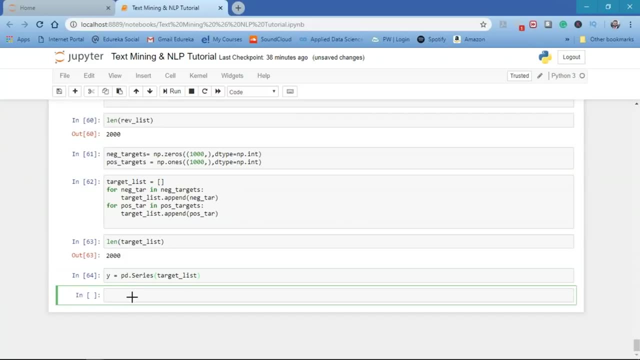 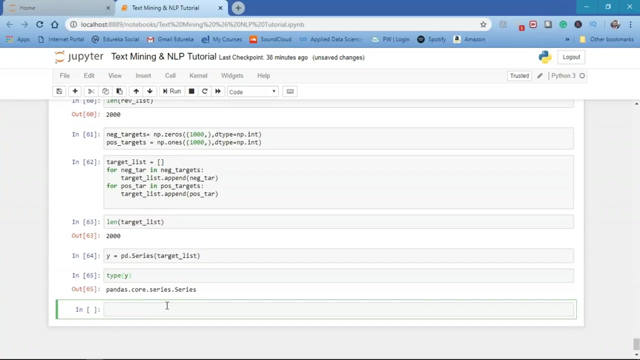 and will add thousand zeros, followed by thousand ones, into the empty list. Now we'll create A panda series for the target list. Now the type of Y must result into a panda series. So if we have a look at the output of the type of Y, 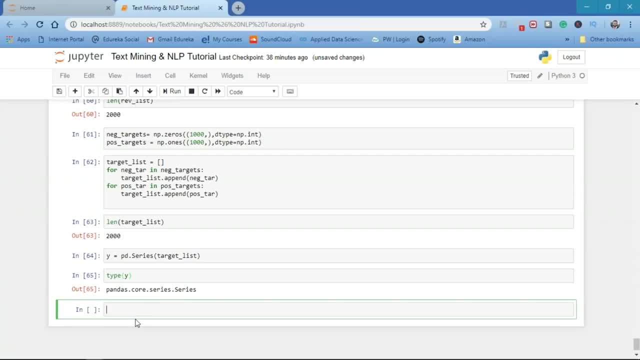 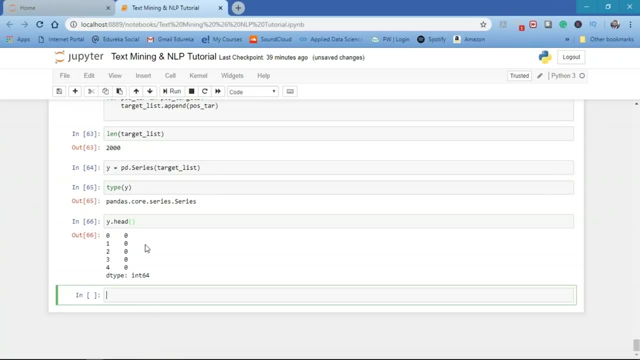 it is pandas dot code or series. that is good. Now let's have a look at the first five entries of the series. So, as you can see, it is thousand zeros which will followed by thousand one. So the first five inputs are all zeros. 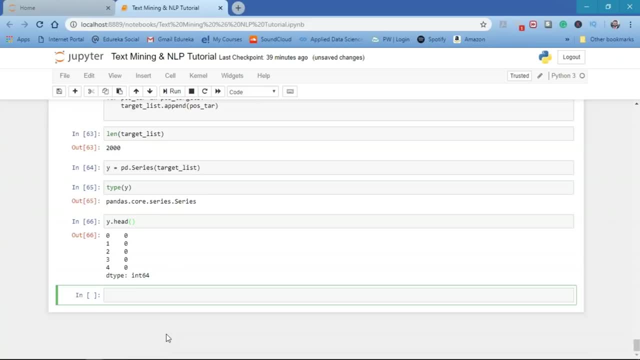 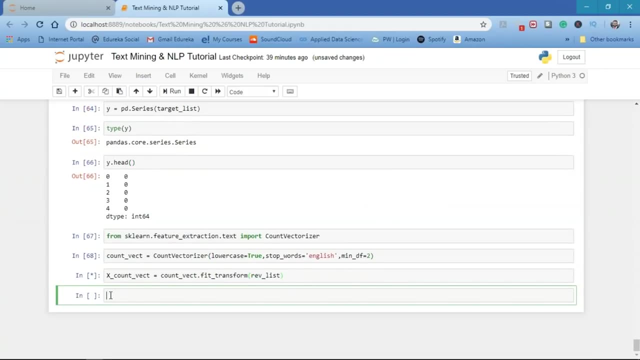 Now we can start creating features using the count vectorizer or the bag of words. For that. we need to import the count vectorizer Now, once we have initialized the vectorizer, and now we need to fit it onto the rev list Now. let us now have a look at the dimensions of this particular vector. 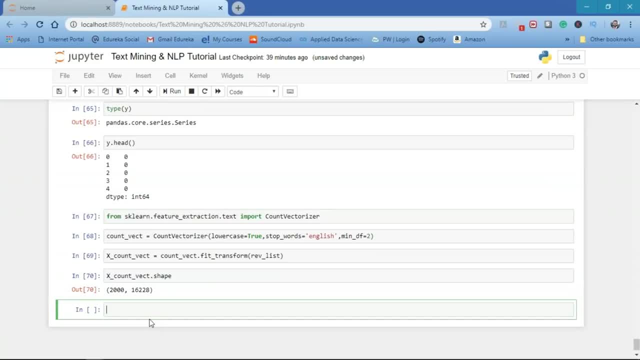 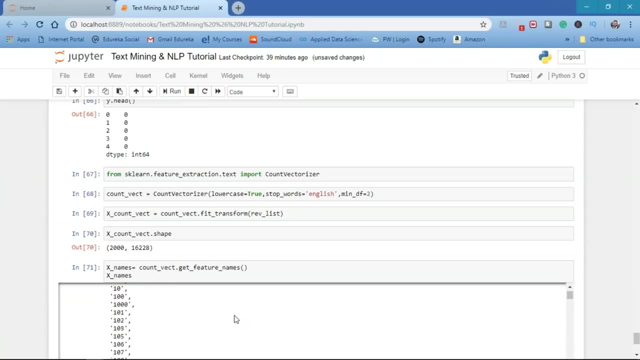 So, as you can see, it's 2000 by 16,228.. Now we are going to create a list with the names of all the features by tapping the vectorizer name. So, as you can see, here we have our list. 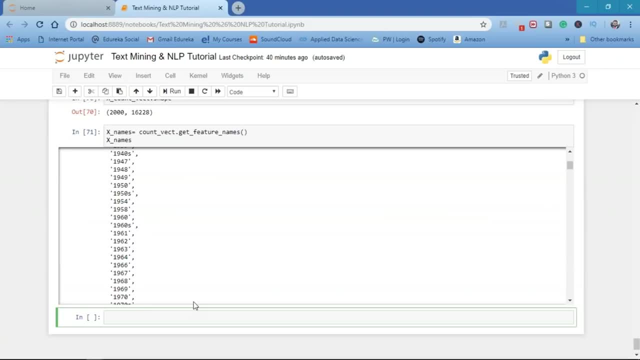 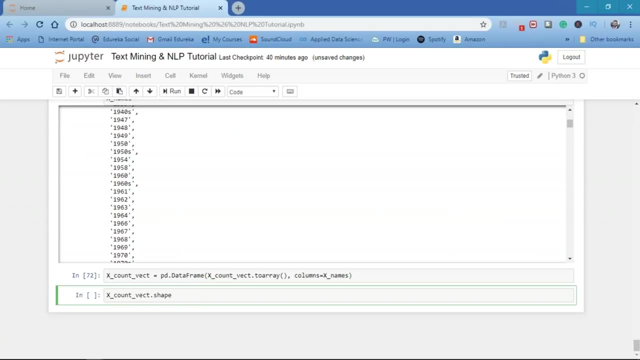 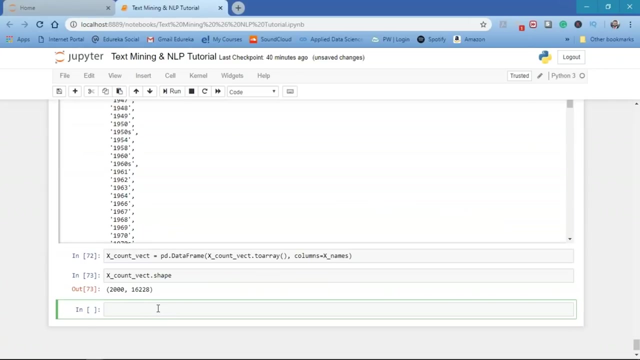 Now what we'll do is we'll create a pandas data frame by passing the sci-pi CSR matrix as values and feature names as the column names. Now, let us now check the dimension of this particular pandas data frame. So you can see, it's the same dimension: 2000 by 16,228.. 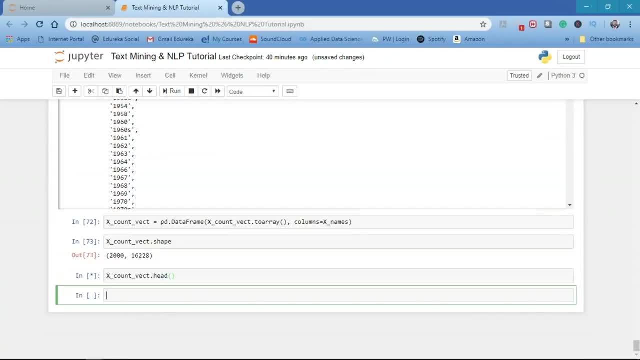 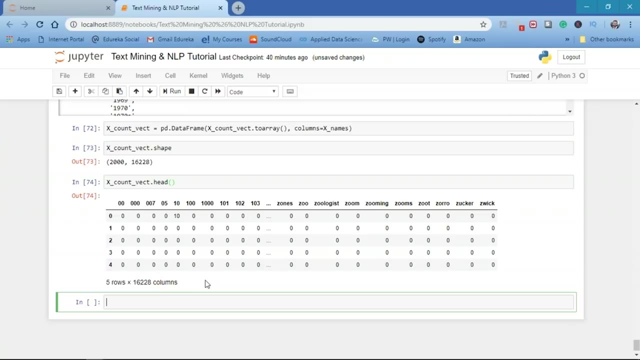 Now, if we have a look at the top five rows of the data frame, so as you can see here we have 16,228 columns with five rows and all the inputs are here: zero. Now the data frame we are going to do is now split it into training and testing sets. 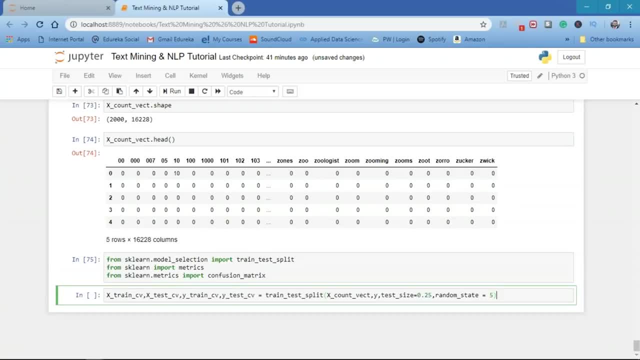 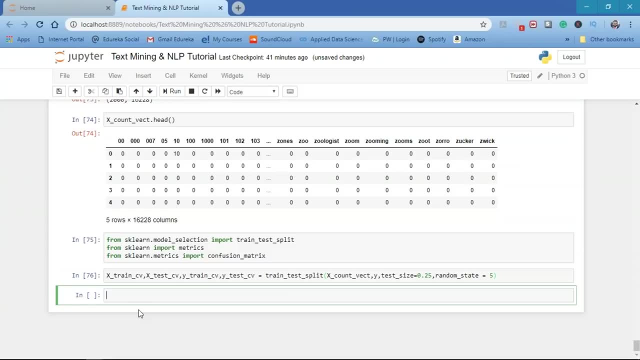 And let us now examine the training and the test sets as well. So, as you can see, the size here we have defined as 0.25.. There's a test set that is 25%. The training set will have the 75% of the particular data frame. 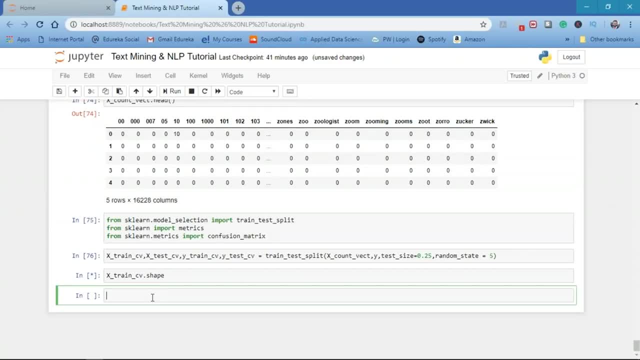 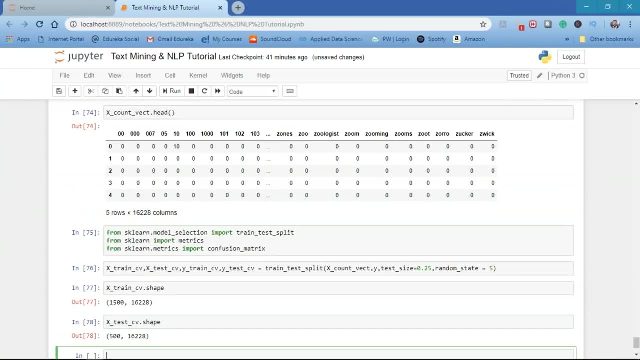 So if you have a look at the shape of the X train, we have 15,000.. And if you have a look at the dimension of X test, this is 5,000.. So now our data is split. now We'll use the naive bias classifier. 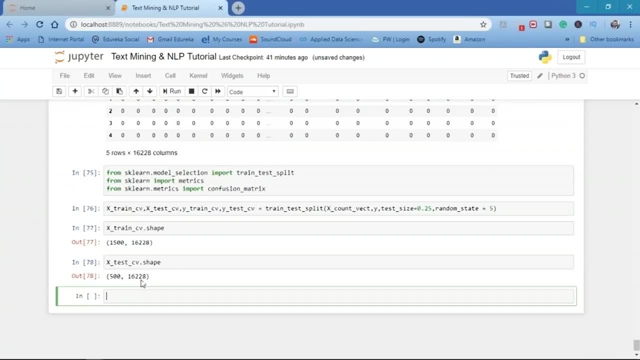 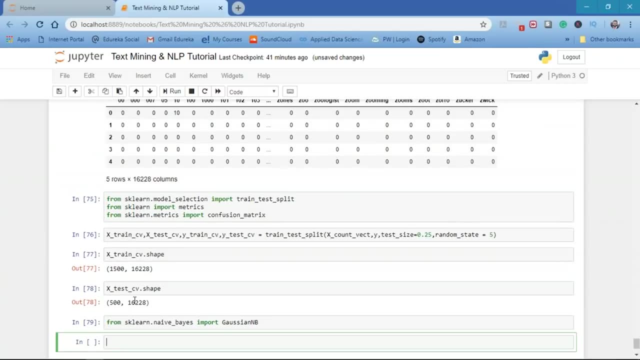 for text classification over the training and testing sets. So now most of you guys might already be aware of what a naive bias classifier is. So it is basically a classification technique based on the Bayes theorem with an assumption of Independence among predictors. in simple terms, a naive bias classifier assumes 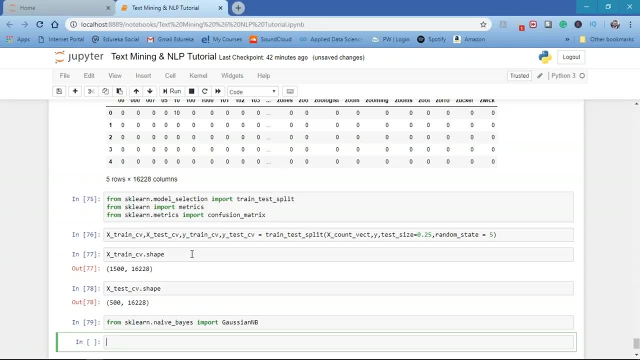 that the presence of a particular feature in a class is unrelated to the presence of any other feature. to know more, you can watch our naive bias classifier video, The link to which is given in the description box below, If you want to pause at this moment of time. 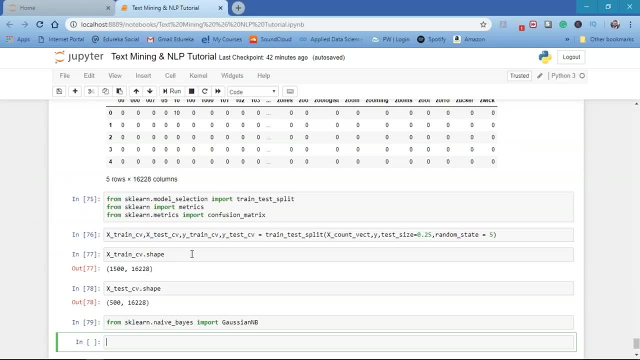 and check quickly what a naive bias classifier does and how it works. You can check that video and come back here now. to implement naive bias algorithm in python will use the following library and the functions: we are going to import the Gaussian NB from SQL learn library. 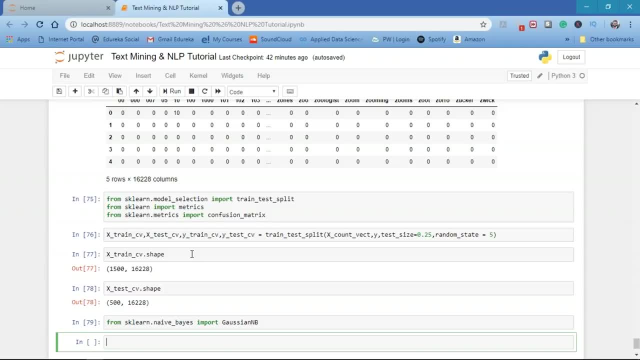 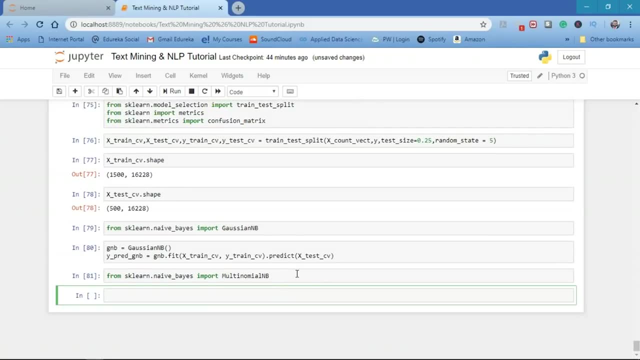 which is a scikit-learn. We are going to instantiate the classifier now and fit the classifier with the training features and the labels. We are also going to import the multinomial naive bias, because we do not have only two features here, We have the multinomial features. 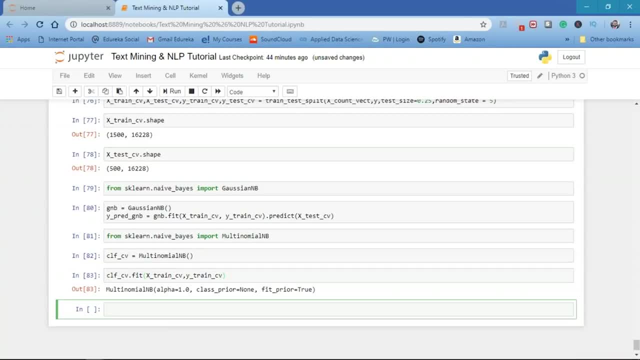 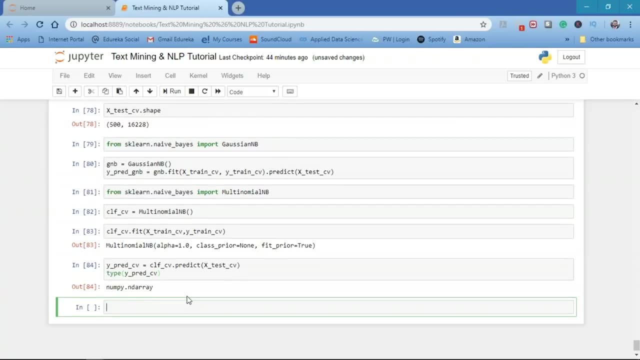 So now we have passed the training and the test data set to this particular multinomial naive bias, and then we will use the predictor function and pass the training features. Now let's have a look and check the accuracy of this particular metrics. So, as you can see here, the accuracy here is one. 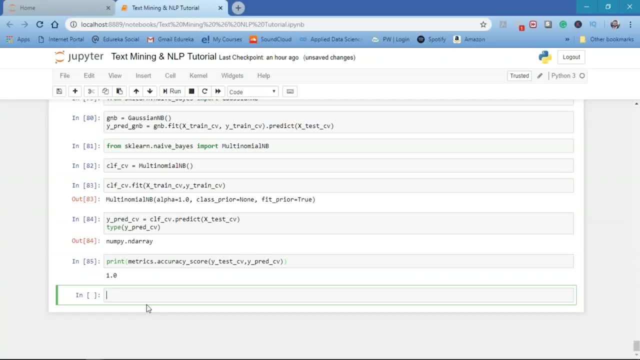 that is very highly unlikely, but since it has given one, that means it is overfitting and it is overly accurate, and you can also check the confusion Matrix for the same. for that, what you need to do is use the confusion and let's go Matrix on these variables. 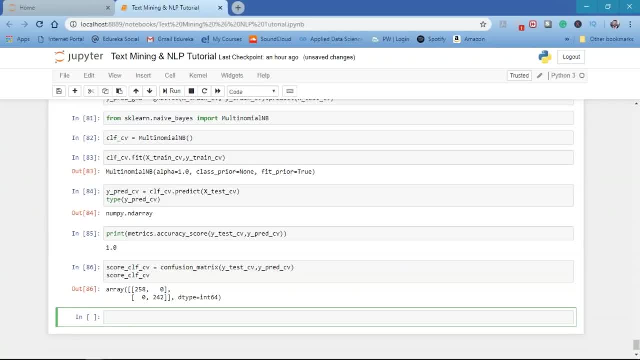 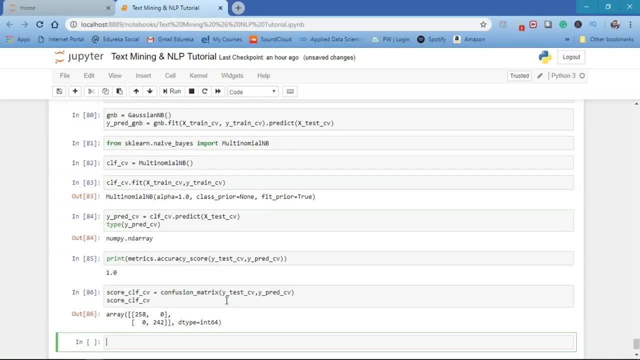 which is y underscore test and y underscore predicted. So, as you can see here, although it has predicted a hundred percent accuracy, the accuracy is one. this is very highly unlikely and you might have got a different output for this one. I've got the output here as 1.0.. 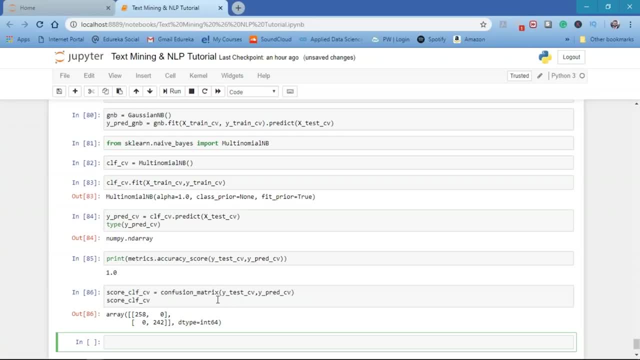 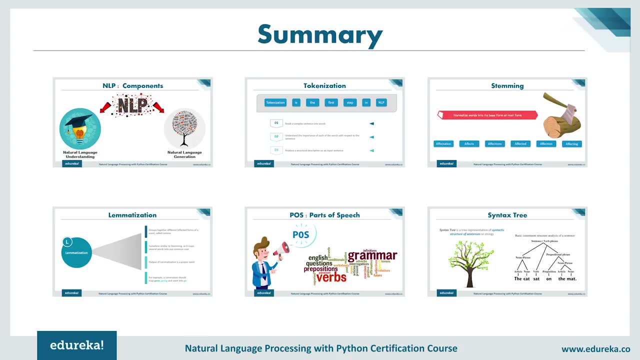 You might have got an output as 0.6, 0.7 or any number in between 0 and 1.. So, guys, this is it for today's session. I hope you understood a lot of things regarding text mining and natural language processing, the tokenization stemming. 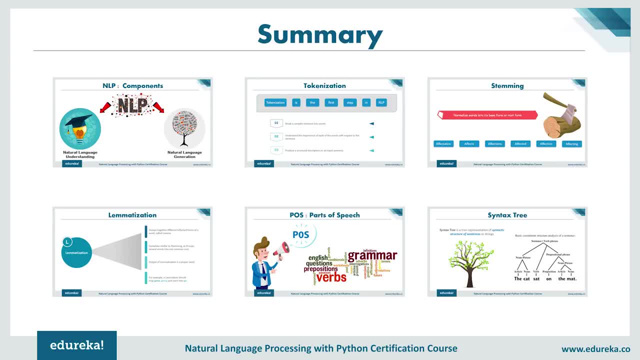 lemmatization: POS taggings, then the name, entity recognition, chunking the syntax- how it is important- the syntax tree, the creation of syntax tree And finally, if you had a look at the final demo here, where we use the naive bias classifier on top of all the NLP operations. 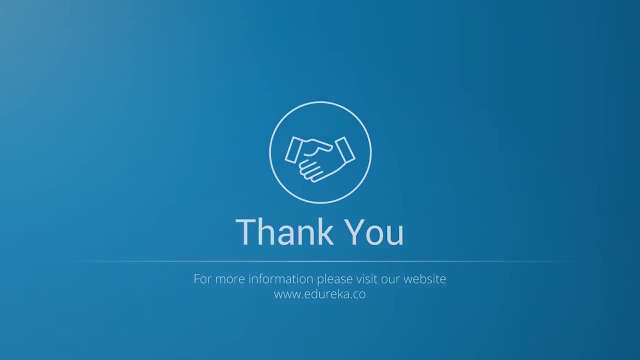 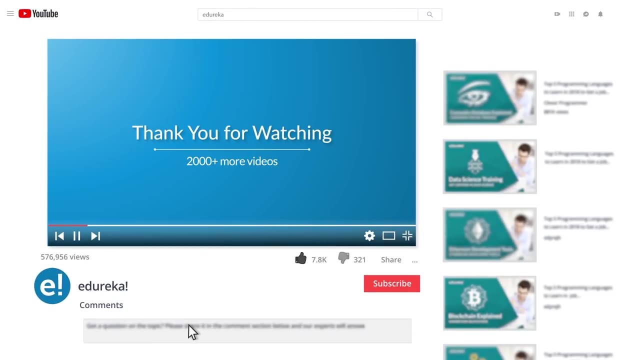 We performed. thank you so much for watching. I hope you have enjoyed listening to this video. Please be kind enough to like it and you can comment any of your doubts and queries and we will reply them at the earliest. Do look out for more videos in our playlist. 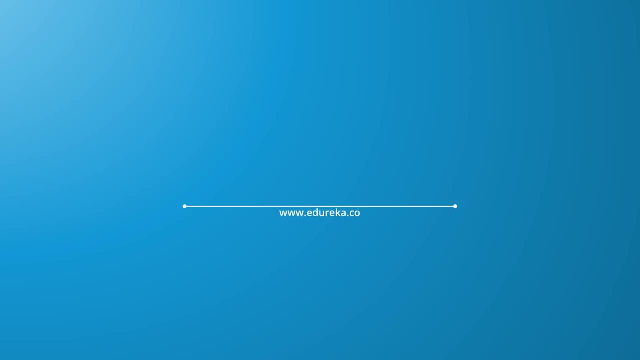 and subscribe to edureka channel to learn more Happy learning. Thank you.